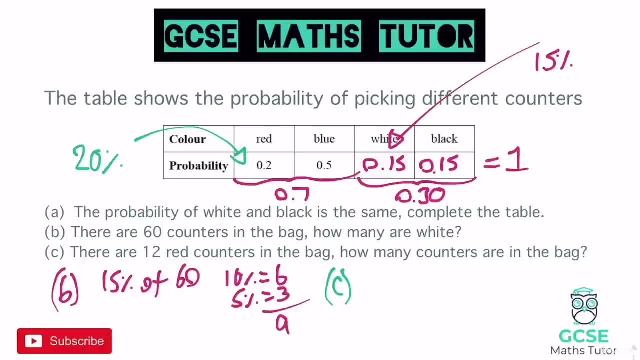 here, which is 20%, is now 12 counters. So all that's actually saying is: 20% equals 12 counters. Now, that's okay. we can turn that back into 100%. quite nice and easy. I could just times that by 5, but let's imagine it's not a nice percentage. I'd have to try and 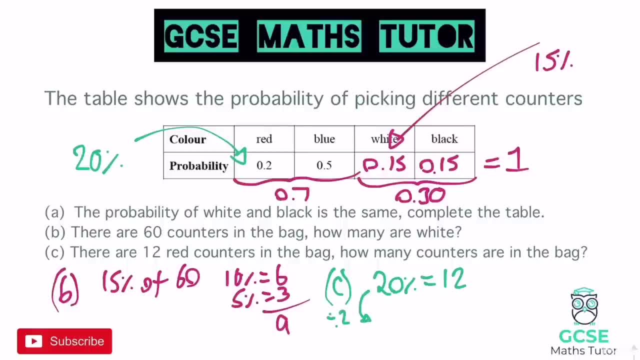 break it down to something which turns into 100.. So we could divide it by 2,, which would give us 10%, which is half of 12,, which is 6, and then times that by 10 to get us back to 100%. 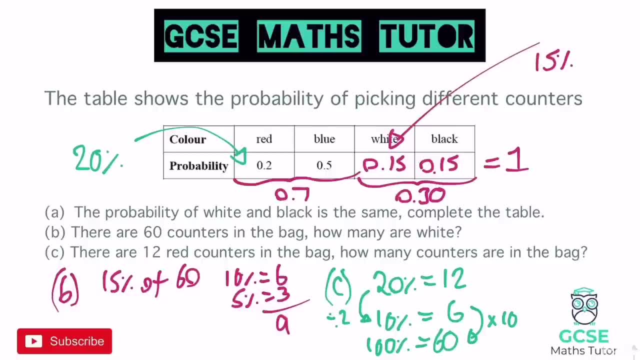 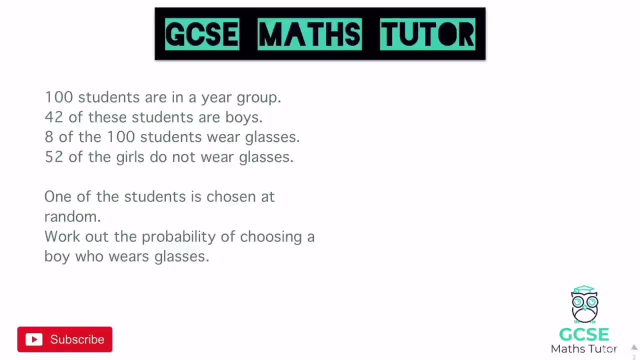 So that's actually just times 20% by 5, but I think that's quite nice just to break it down and build it back up. so 60 counters there would be in the bag. Okay, so we've got a lot of information here. 100 students are in a year group and then 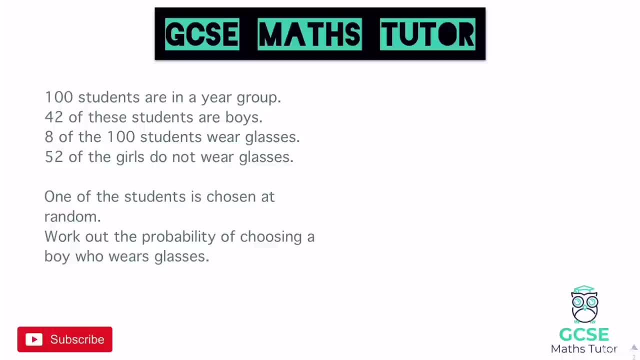 we've got some information about whether they wear or do not wear glasses. It wants us to work out the probability of choosing a boy who wears glasses. When you've got a lot of information like this, I like to organise it in a two-way table, So I'm going to put. 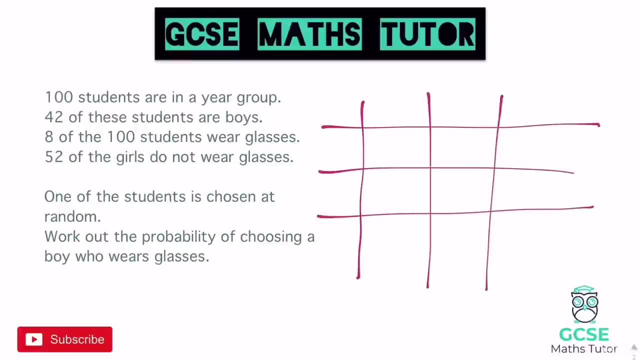 this all into a two-way table. Again, you could use a frequency tree, but I'm just going to opt for using a two-way table And girls on the side. again, you could have them at the top, but I'm going to put them. 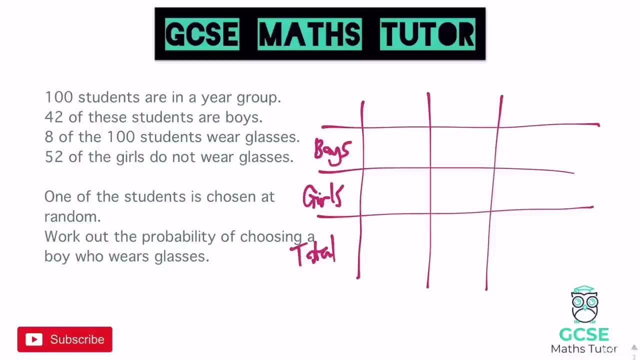 to the side, And then you've got a total down the bottom. And then we've got whether they wear or do not wear glasses, And again we've got a total here. So what I'm going to do is put the numbers within the question. We've got 100 students in the year group, 42 of 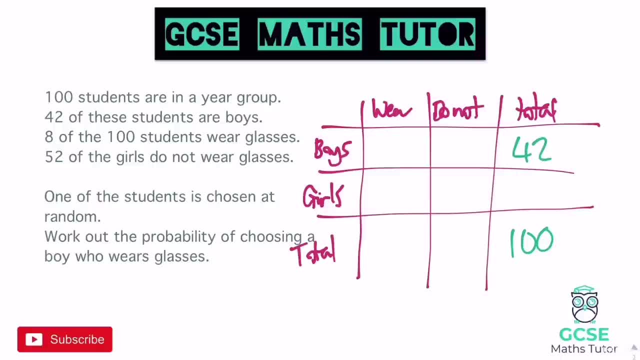 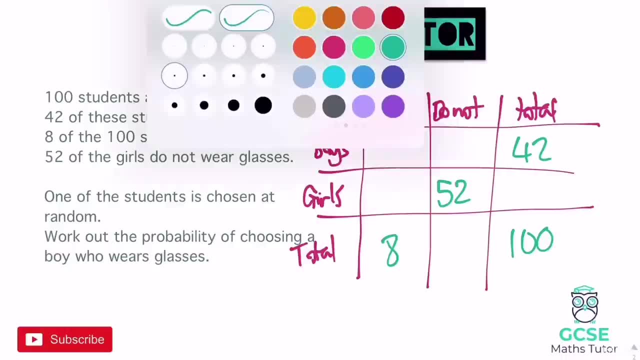 them are boys. 8 out of 100 students wear glasses, so 8 students here wear glasses and 52 of the girls do not wear glasses. so 52 just here. That's everything in the question. we've just got to fill in all the missing numbers now. So if there are 42 boys here, 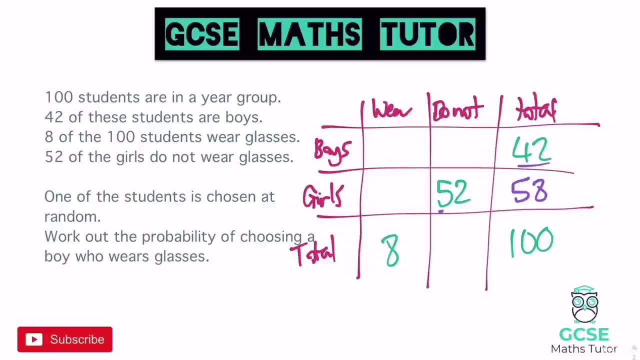 that must mean that there are 58 girls And out of those 52 do not wear glasses. so that must mean that 6 of them do. Now again we've got 8 that do wear glasses. 6 of them are. 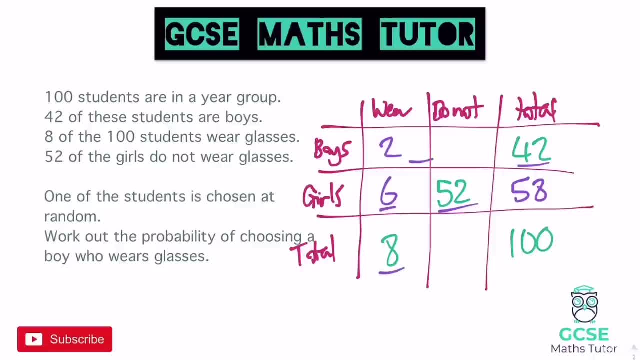 girls, so 2 boys must wear glasses. And again, going along this way, that has to add up to 42,, so that must be 40. And then moving downwards or across from another direction, I could add those together to make 92.. And a very quick check here: those two add up to 100,. 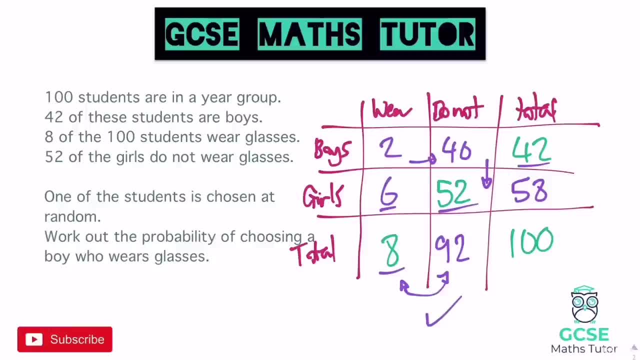 so that's right. we're happy with that. Now it says: work out the probability of choosing a boy who wears glasses, and one of the students is picked at random while two of the boys wear glasses, So that would be 2 students. 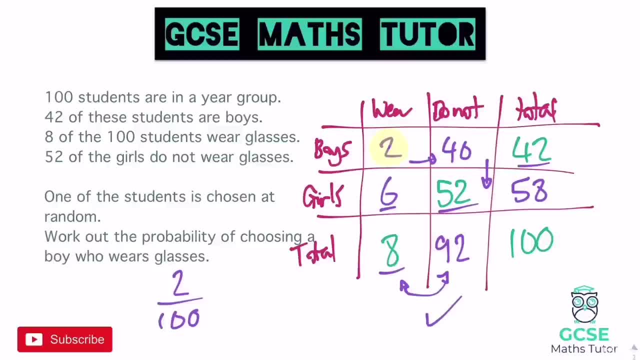 out of the 100 students that we've got here. You don't have to simplify that, but just a quick note. it could have said in the wording here it could have said, rather than saying one of the students, it could have said one of the boys. Now, if it had said it, maybe 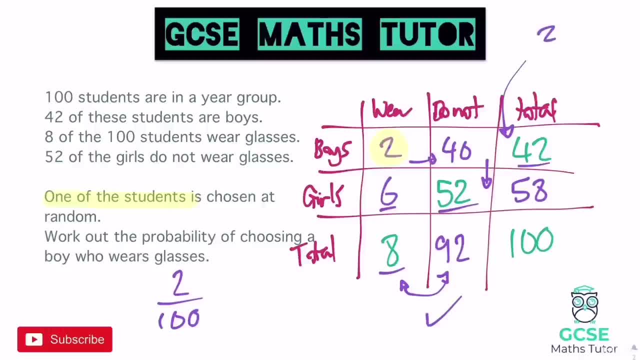 it had picked one of the boys, then that would have been out of 42, so it would have been 2 over 42. So that's what the wording says. so it does say one of the students. it doesn't dictate whether it's boys or girls, so it's out of 100.. 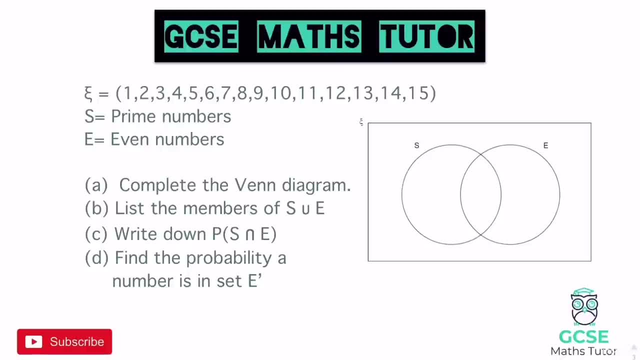 And moving on to a Venn diagram. now, this symbol here just means all the numbers that we're going to put into the Venn diagram. so we've got the numbers 1 to 15, and then it says prime numbers and even numbers. Now, what I'm going to do is I'm going to write. 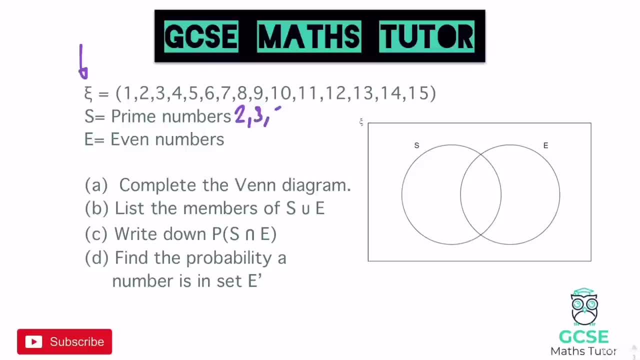 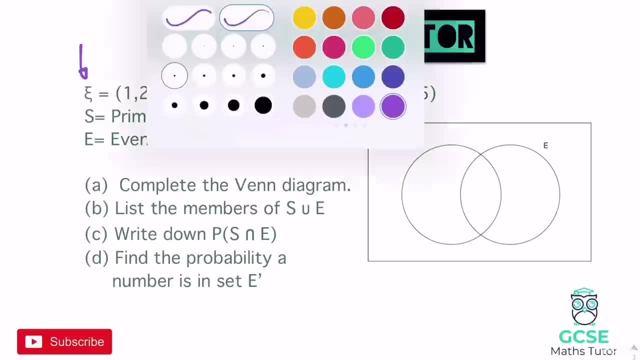 down the prime numbers to start with. so we have 2,, 3,, 5,, 7,, 11 and 13. And we could write down all the even numbers as well, but I'm hoping we can recognise them quite easily. 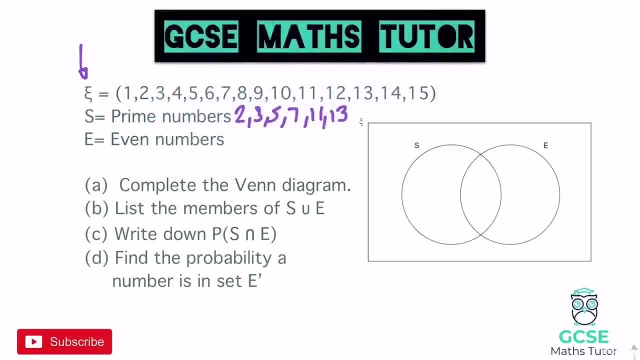 Now what I'm going to have a look at is which numbers are in both. Now, the only even number in that prime list is the 2, so that's going to go in the middle because that says it's in both. so I'm going to cross the 2 off and 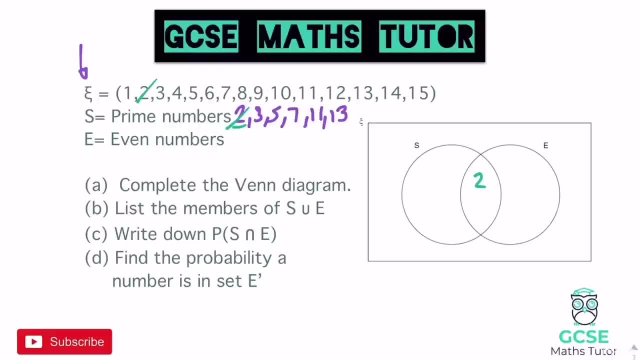 cross it off from the main list. It then says: obviously we've got the prime numbers in set S, so I need to put all the rest into set S, so 3,, 5,, 7,, 11, 13.. Again, I'm going to. 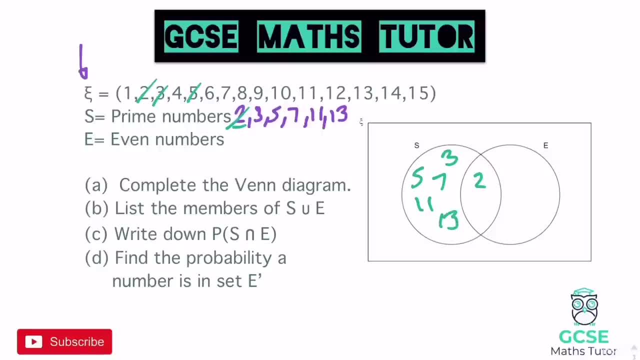 cross them all off from the main list. so 3,, 5,, 7,, 11,, 13.. And then all the even numbers are going to go in the right circle there. so we've already got rid of 2,, so 4,, 7,, 11,. 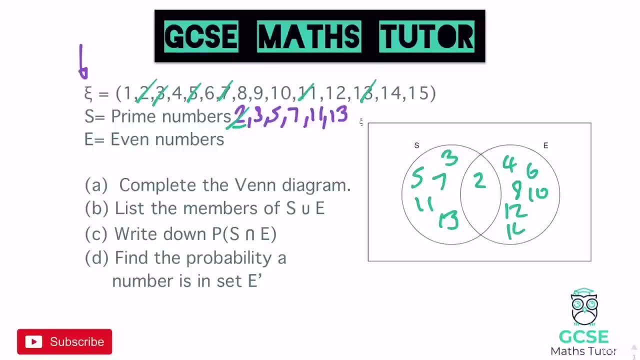 6, 8,, 10,, 12,, 14.. And again, just crossing those all off from the main list, So 4, 6,, 8,, 10,, 12,, 14.. And the remaining numbers there are going to go round the outside. so I've 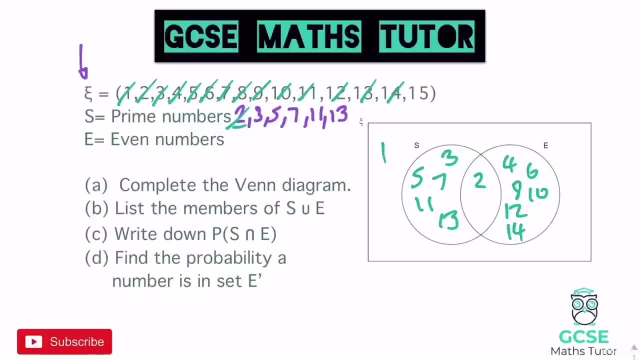 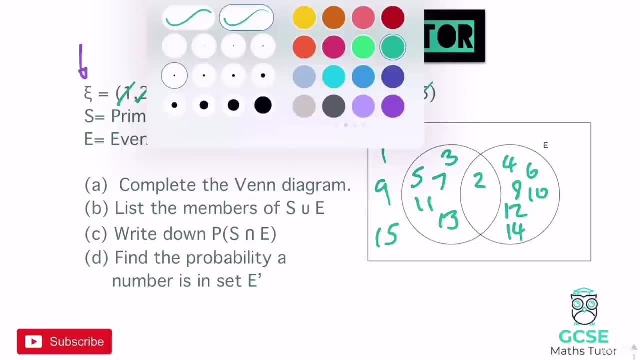 got: 1, cross that off, stick it on the outside. 9, cross it off, stick it on the outside. and 15, cross that off and stick it on the outside. Now we're asked some questions about the Venn diagram. It says: list the members of S? U E Now that U stands for the Union. 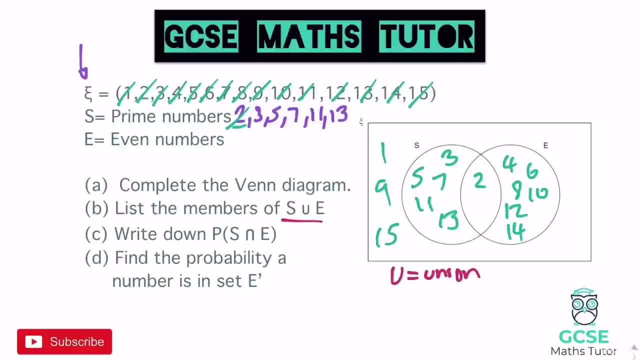 and the Union is everything within the circles. So that's the members of S, the members of E and that number in the middle there. So if I write them all down, all the numbers there for part B are from left to right. we've got 5,, 11,, 7,, 3,, 13,, 2, and all those. 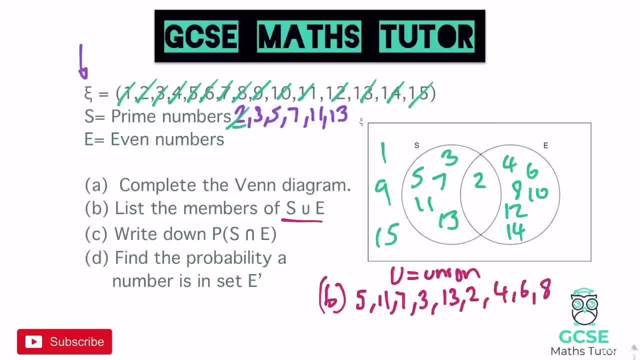 even numbers 4,, 6,, 8,, 10,, 12, and 14.. Let's have a look at part C. Write down P, S, N, E, Now that P at the start there just stands for probability. So write: 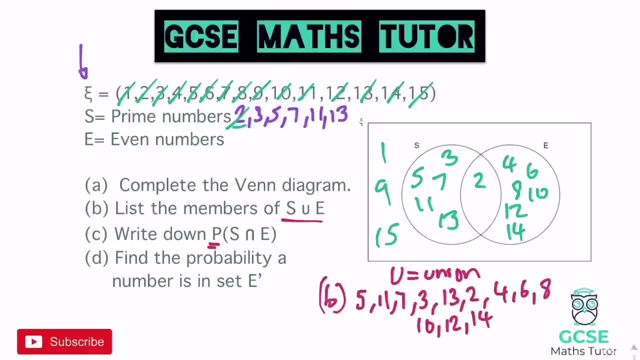 down the probability that it's in S, N, E. Now that N is a different symbol again and the N stands for the intersection. So this is asking me: what's the probability of picking the number that's in the intersection? Now, in the intersection we only have this number. 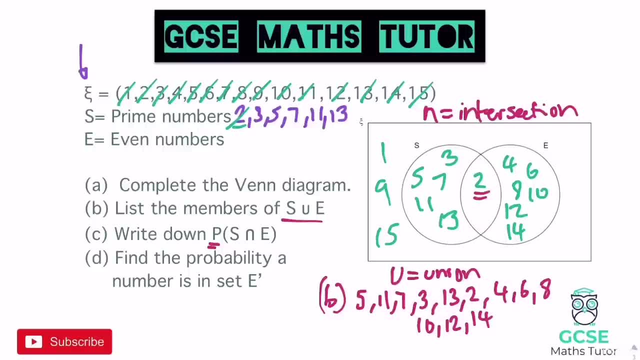 2. So there's one number. so for that part C, there I'd say one number out of because it's a probability and there are 15 numbers in the intersection. So that's the probability In total. So the probability there would be 1 out of 15. for part C, Again, it could 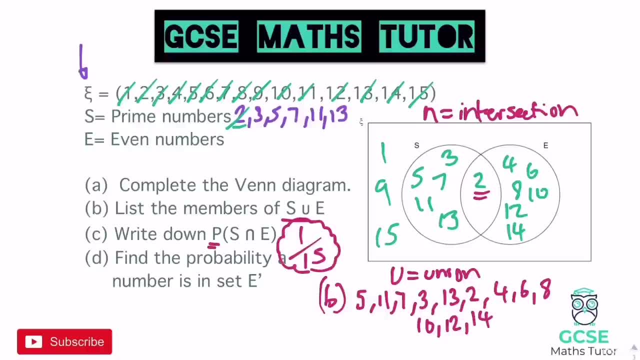 say S, U, E, and that would be again. we've got to count all the numbers in the union. Let's have a look: There's 3,, 6,, 9,, 12 numbers there, so that would be 12 out of 15.. Now 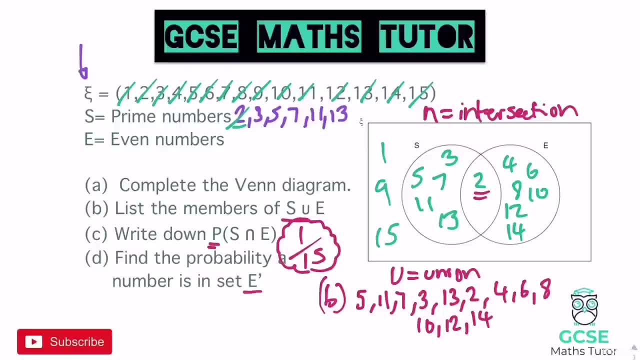 the final part. here it says: find the probability. a number is in set E dash, And that little dash just means not in. So E dash means not in E. So E dash, not in E. Now if we have a look We've got quite a few numbers that are in E. So all of these numbers here are in E. 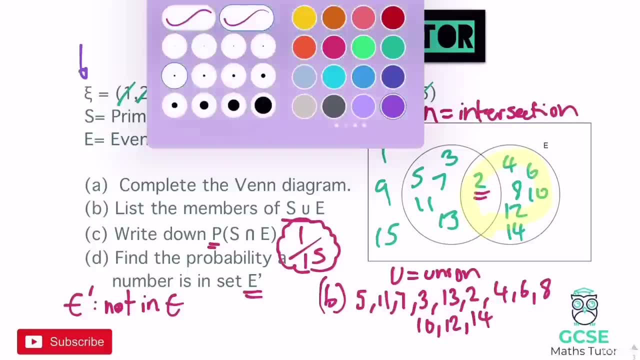 So all we need to do is have a look at how many numbers are not in E. So let's pick a different colour. Let's underline all the numbers that are not in E: 1,, 2,, 3,, 4,, 5,, 6,. 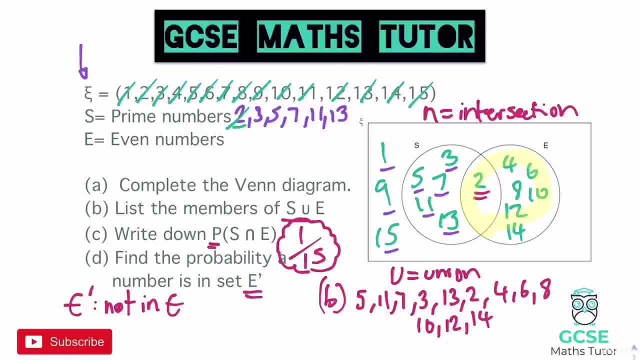 7, 8.. So the probability of picking a number that's not in E is 8, again out of 15.. So again, just remember that the little dash means not in that set, The N means the intersection where they cross over And the U stands for 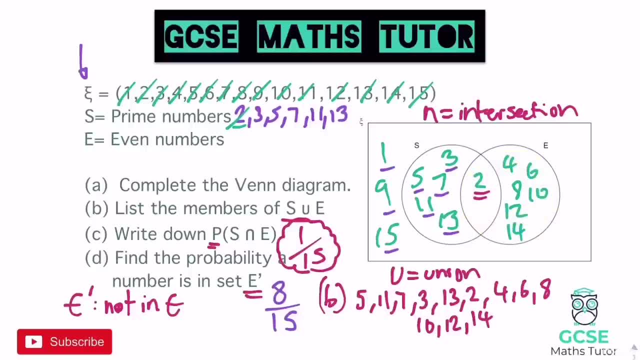 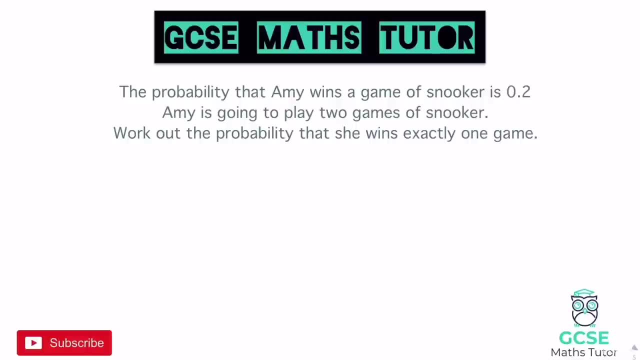 The union, which is all the numbers within all of the circles. OK, so the probability that Amy wins a game of snooker is 0.2.. Amy's going to play two games of snooker and work out the probability that she wins exactly one game. Now let's. 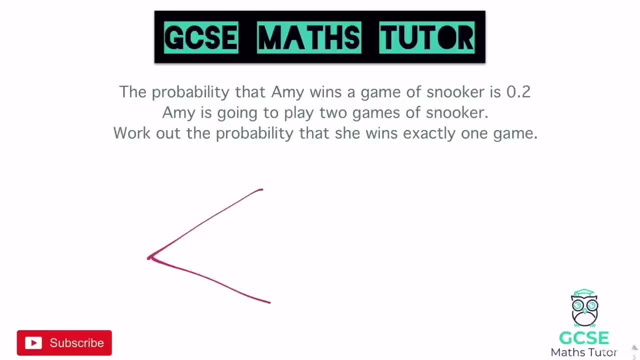 have a look at this one. So if we create a probability tree for this, we've got on the first game, which I'll label this branch as the first. she either wins or she loses, And the probability that she wins is 0.2 and the probability that she loses is 0.8.. Now she's. 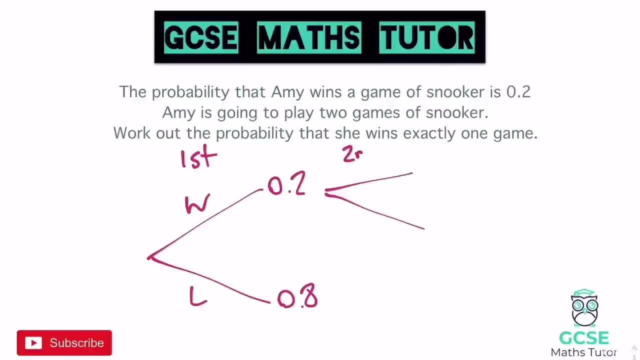 going to play a second game, So we've got a second branch again. this is after she's won, and we've got a second branch here in case she loses. But again she wins, or she loses, and she wins or she. 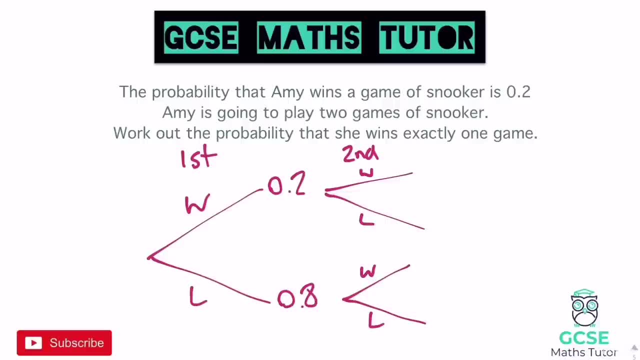 loses. Now it doesn't say the probability changes on the second game, so it's all just going to be the same- 0.2 for a win, 0.8 for a loss and the same below 0.2 for a win. 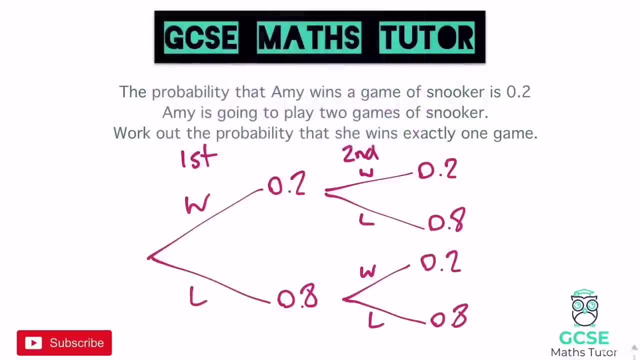 0.8 for a loss. OK, So it says: work out the probability. she wins exactly one game. So she wins exactly one game. That's quite important there. Now, the only way that she wins exactly one game is if she also loses a game. so this win-win up here is no good, and this 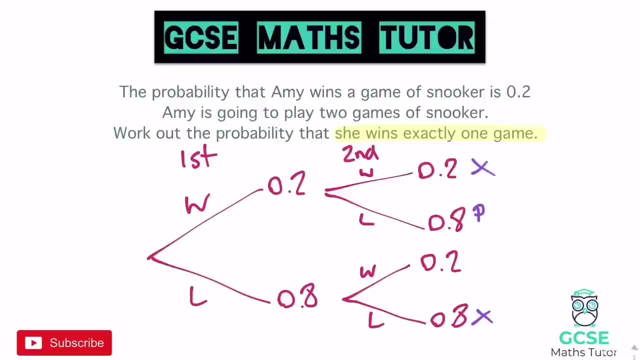 lose-lose down here is no good. But here we've got the probability of a win and then a loss, And then here we've got the probability of a loss and then a win, And what we need to do is work out these two probabilities. So to get to this second branch here, if we 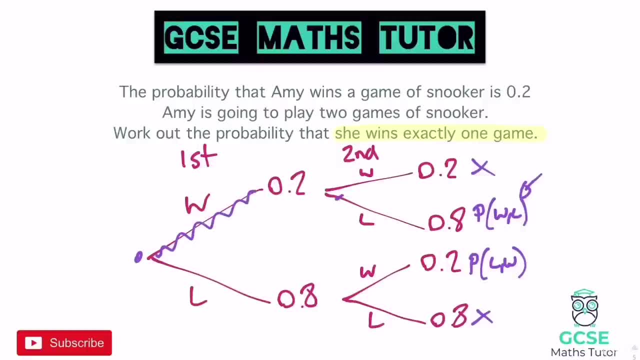 go to the start. we go up through the win and down through the loss. So that's 0.2, multiplied by 0.8.. And 0.2 times 3.8? 0.8.. times 0.8 is 0.16.. Looking at the second option there, she could lose and then win, And that just. 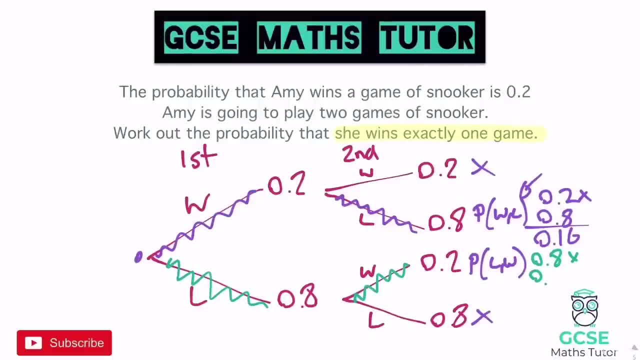 goes through 0.8 multiplied by 0.2, which gives us the same answer there of 0.16.. So we've got our two answers there. We've got 0.16 for that route and 0.16 for that route, And when we've 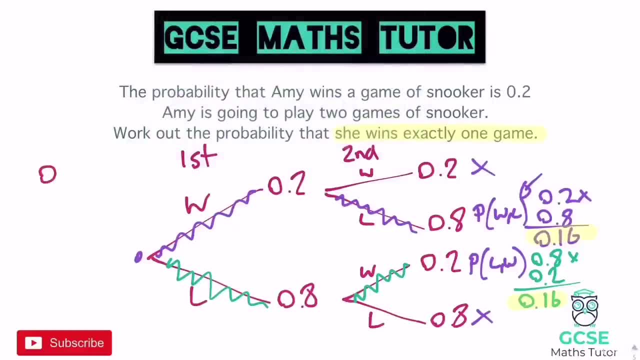 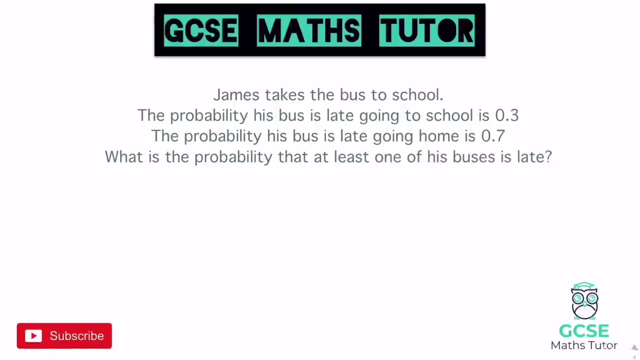 got two probabilities to combine. we just add them both together. So 0.16 add 0.16 gives us a total probability there of 0.32 as our final answer. So another probability question: James takes the bus to school. The probability his bus is late going to school is 0.3 and the probability 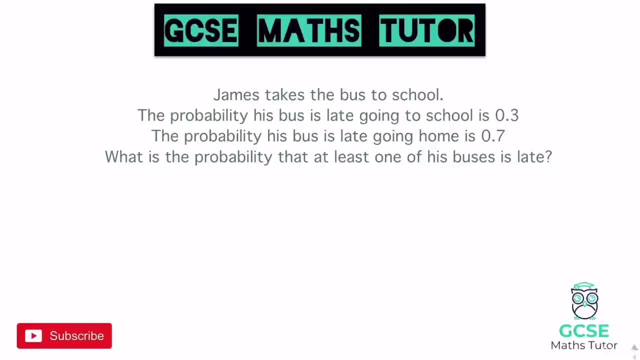 his bus is late going home is 0.7.. What is the probability that at least one of his buses is late? Let's have a look at creating a tree. So this time it's not the same thing on both occasions. We've got one where he's going to school and the other part of the branch is where he's going home. 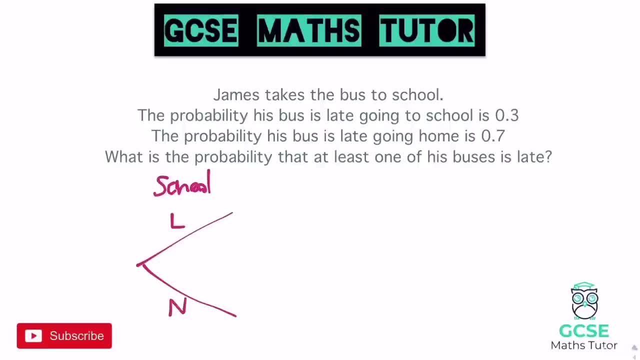 But when he goes to school it's either late or he's late. So we've got one where he's going to school and the other part of the branch is, or it's not, late, And the probability of late is 0.3.. So, therefore, the probability that it's not 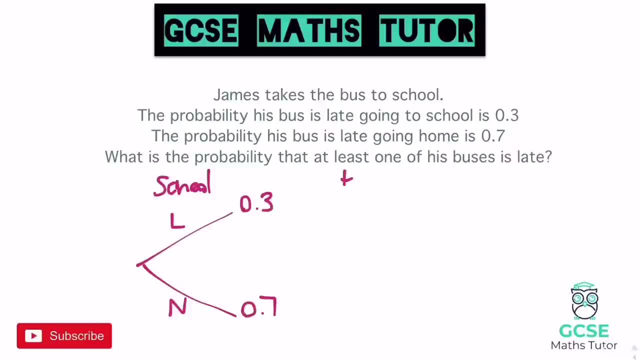 late is 0.7.. Then we've got the next branch, which is going home. Now the numbers look quite similar here, because we've got 0.7 in. there again We've got late and not late, And again late and not late, But this time it says going home, the probability is late is 0.7.. So this 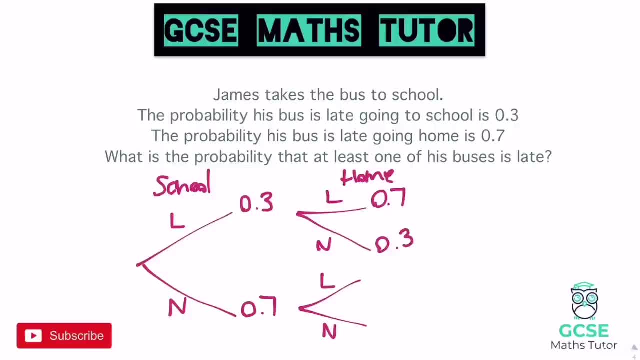 would be 0.7 and again 0.3 and the same below. So 0.7 and 0.3.. Now the question says to work out the probability that at least one of his buses is late. So this time it's not just one. 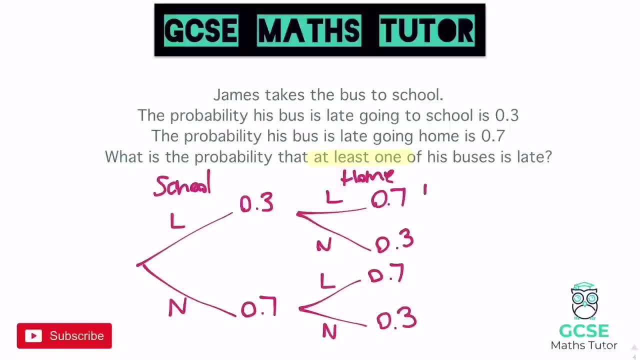 late. it could be late on both, So we could have the probability. let's do this in a different colour. We could have the probability that it is late and then late. We could have the probability that it is late and then not late. That's at least one, And the probability that it is not late and 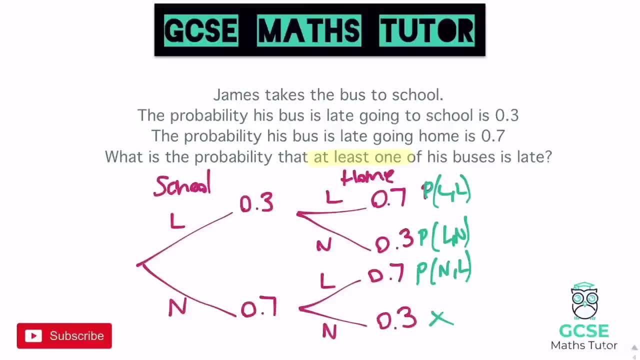 then late on the second one, But not late on both is no good to us, So we don't want that one. So what we need to do is work out these three probabilities: this time So late, then late goes through 0.3 and then 0.7, which is 0.21.. We've got the probability of it being late, then not late. 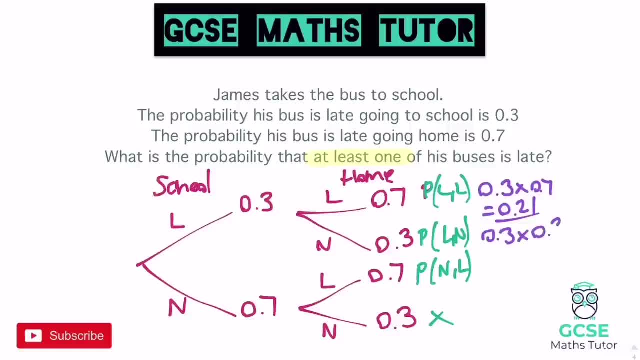 which is 0.3 times another 0.3,, which is 0.09.. And we've got that third one there, okay, which is not late, and then late, which is 0.7 times 0.7.. And that equals 0.49.. 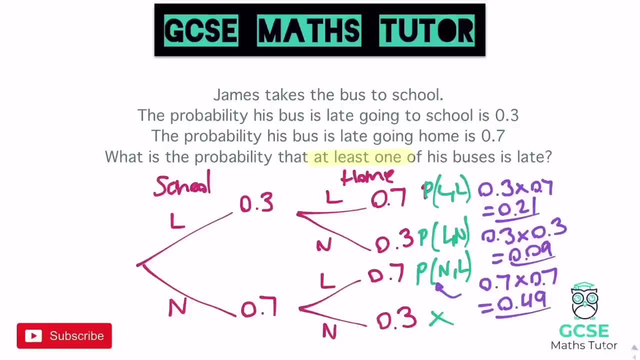 So this time we've got three probabilities to add together, But because we've got a combination there again, we just add them all up, So 0.21, 0.09 and 0.49.. And all together that adds up So. 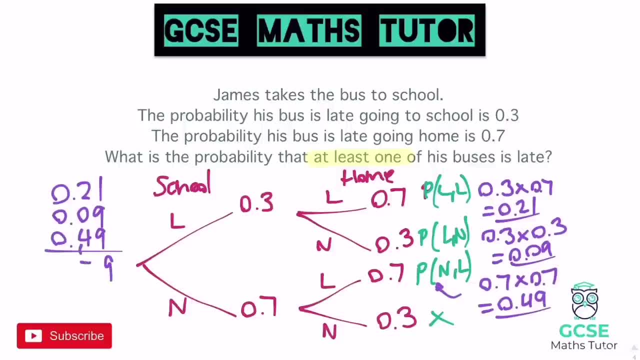 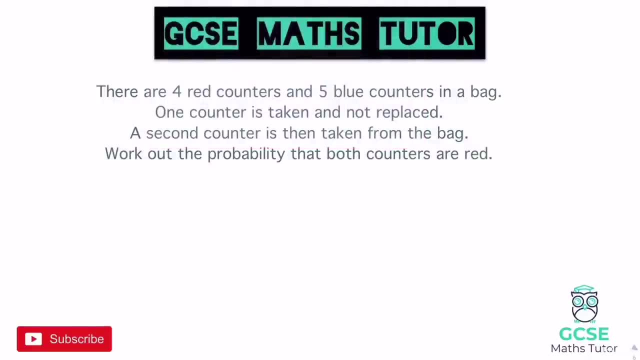 let's have a look: 8,, 9, carry the 1,, 4,, 5,, 6,, 7.. So 0.79 is our final answer for this one. Let's have a look at some with some fractions. Okay, so the hardest one out of the bunch here. 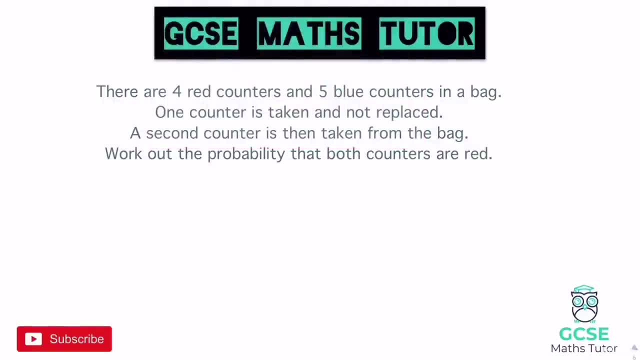 we've got four red counters and five blue counters. One counter is taken and not replaced, And then a second counter is taken from the bag. Work out the probability that both are red. Now, this piece of language here is important. Taken and not replaced, So that's going to give us. 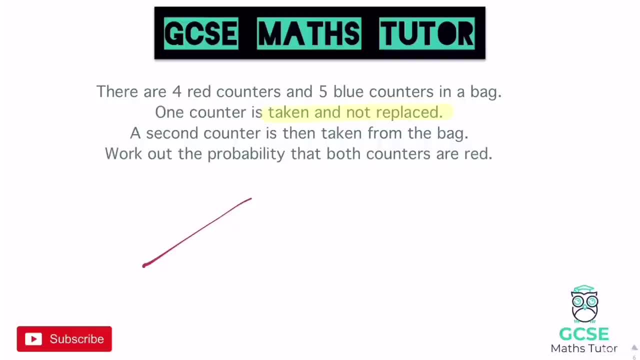 two options here when we do our tree. But let's have a look at the first option. So initially we've got red or blue. This is our first pick. And the red counters- there are four out of a total of nine, And the blue- there are five out. 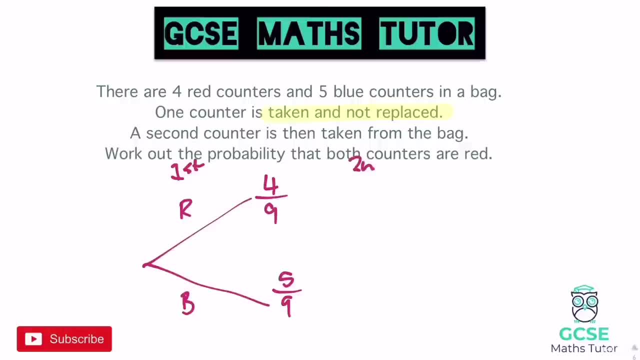 of a total of nine. Now let's just have a look at this second pick to start with, And let's imagine we took a red. So if we take a red, what have we got now? We've got three reds left in the bag And there are only eight counters in total, But none of the 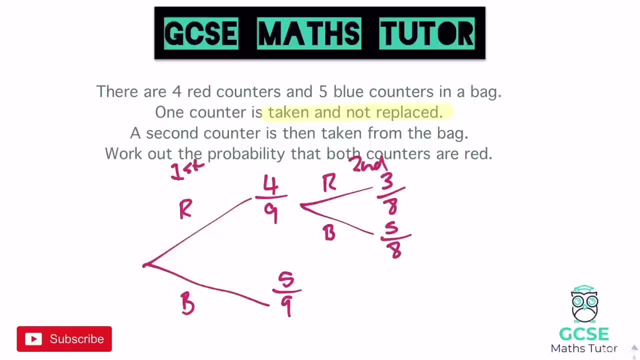 blues were taken, So we still have five And that balances out to eight there on the bottom. So we've got that option there Now, because this is going to be different: taken and not replaced. the second part of the tree is now going to be different, Because if we go back to the start here, we've 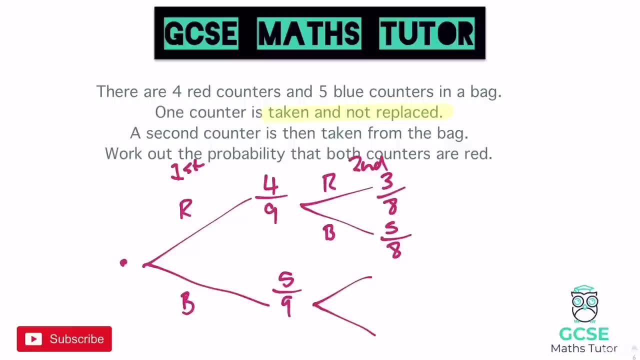 now got to imagine: okay, well, what happens if we took a blue? Well, we still have the option of taking a red or a blue, But this time the blue has been reduced to four. So still out of eight now, But it's going to be four for blue. 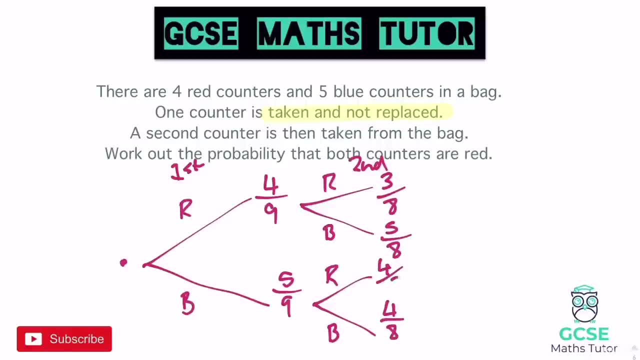 So if we take that out, there's still four reds in the bag. So we've got four out of eight this time for the reds. Now we've got an easier question for this one, because it says: work out the probability that both 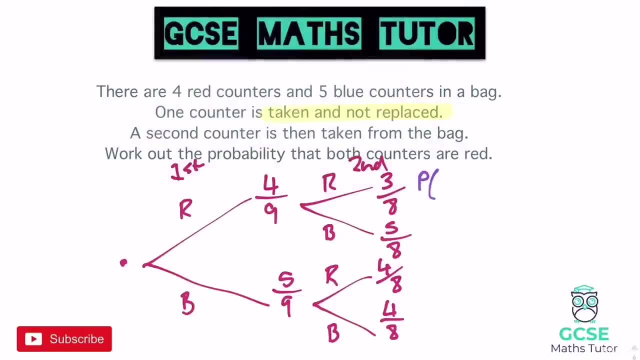 counters are red. Now that gives us only the option of having this branch here, the probability of a red and then a red. And to get that root there we just go through red on the first root and red on the second root, And that gives us four, ninths. And again we multiply, Multiply by three, eighths Times in. 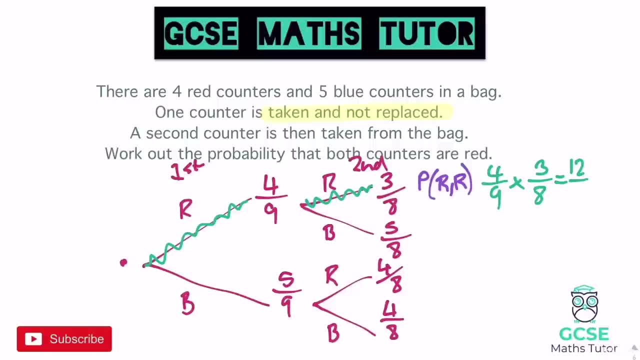 the top gives us 12. Times in the bottom gives us 72. So our final answer there would be 12 out of 72.. Again, though, if we were asked different questions, we would work out multiple roots and we would add them. 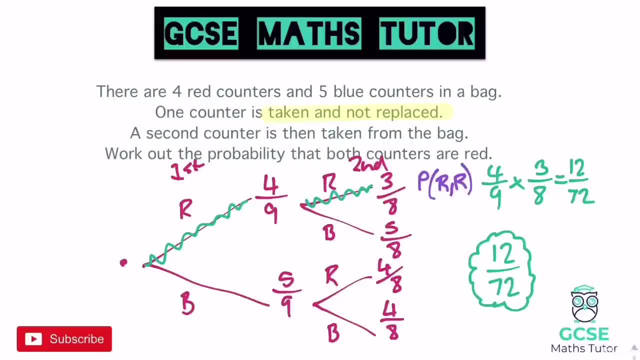 together All the fractions here are going to be out of 72, because the denominators are always going to be nine times eight. So our fraction is going to be nice and easy to add together. If we imagine that it said probability of getting two reds or two blues, the probability of two blues down here would be five times. 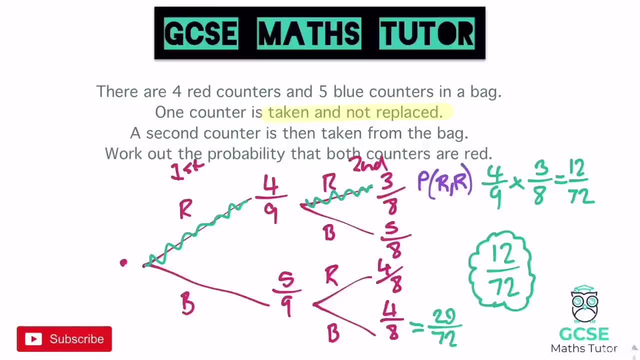 four, Twenty Over 72. And that's nice and easy to add to 12 over 72, because you just have those numerators together. But it's the same process: multiplying across the tree and then adding to combine the probabilities at the end. 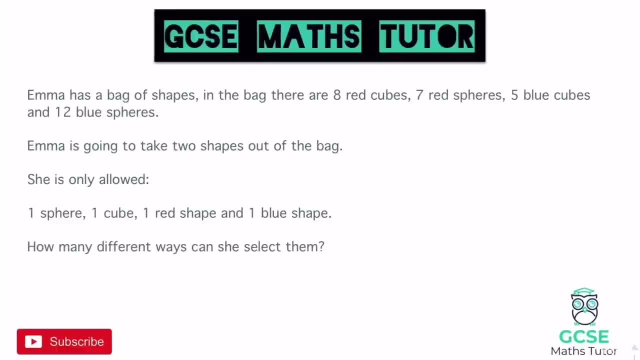 OK, so moving on to probability, So we've got here. Emma has a bag of shapes and in the bag there are eight red, seven- sorry eight- red cubes, seven red spheres, five blue cubes and 12 blue spheres. Emma's going to take two shapes out of the bag and she's 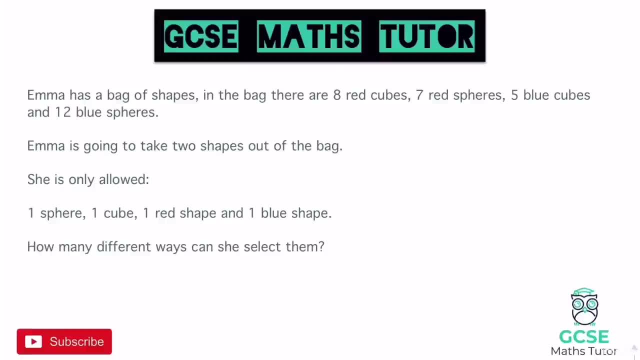 only allowed one sphere, One cube, one red shape and one blue shape. How many different ways can she select them? So look at the product rule for counting here in combinations. So we have to do is think about here: How many options does she have on the first pick? And we're going to multiply it by the amount of 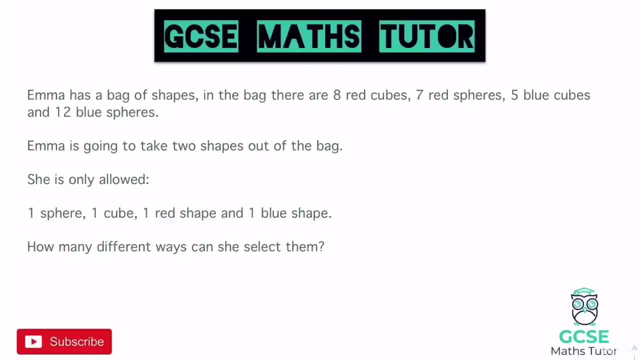 options. on the second pick, Problem is we've got this scenario here where she's only allowed one of each shape and one of each colour. So if we think about this at first, if she takes a red cube, then she can't take another red shape, So she can't take any of those red spheres and she also can't take any of the blue spheres. 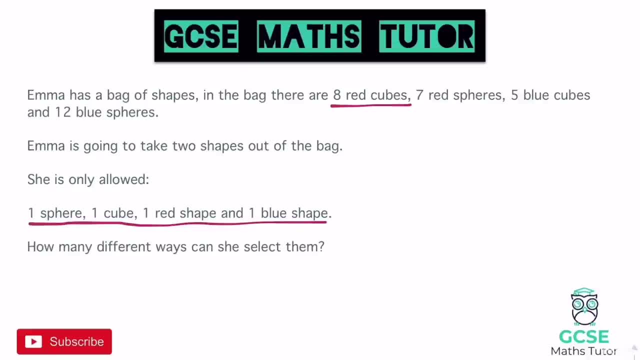 She can only take one of the blue cubes because she's only allowed one red shape and one cube. So if she takes a red cube, the only other option on the next pick is to take a blue sphere. So for that first option there, 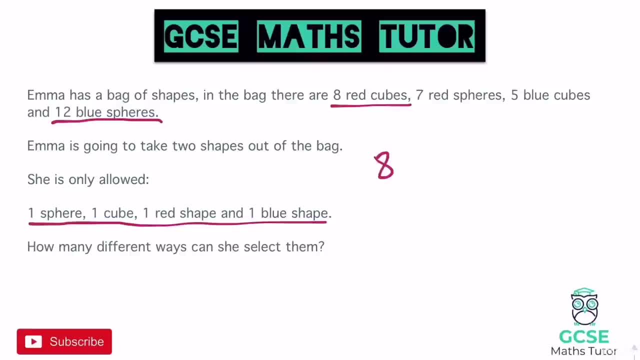 she has eight on the first pick out of the red cubes, multiplied by 12 of the blue spheres. So eight times 12 would give us the amount of combinations there that she can get for the first pick, And that's going to be 96.. So she could take that combination there of red cube and a blue sphere. 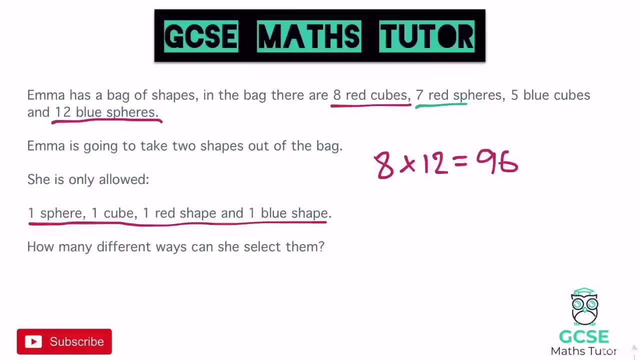 Alternatively, she could also take on the first pick. she could take a red sphere and that would mean on the next pick she can only take a blue cube, to enable her to only have one of each shape and one of each colour. So that would give her a total amount of combinations there of 7 on the first pick there, if we took a red sphere, multiplied by 5 of the blue cubes, and that would be a total of 35.. 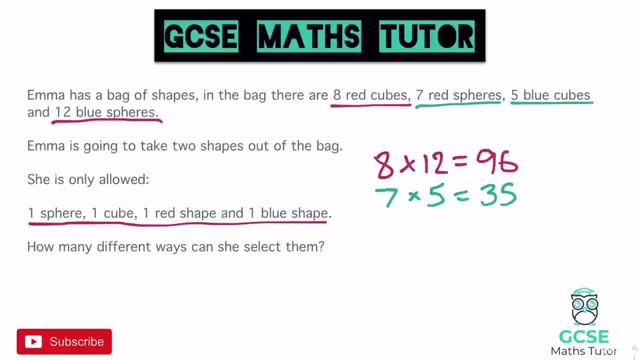 So she has two different ways of picking these shapes. We've got 96 options on the first and 35 on the second. So if we add all these different options together, 96 plus 35 would give us a total amount of combinations here of 131 to meet that criteria of only having one shape and one of the colours for each one there. 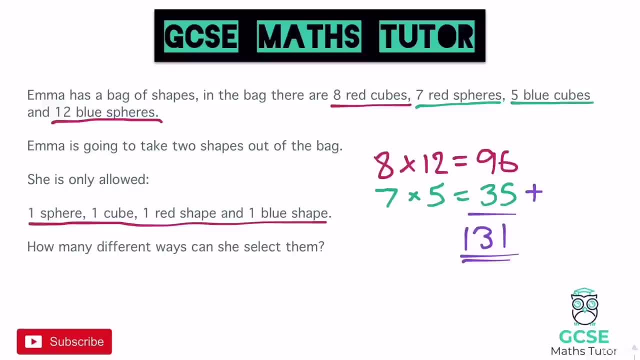 So one sphere, one cube, one red shape and one blue shape and that's combinations there. You've just got to remember how many choices are there on the first pick and you multiply it by however many choices there are on the second pick and then combine any if there are multiple different ways. 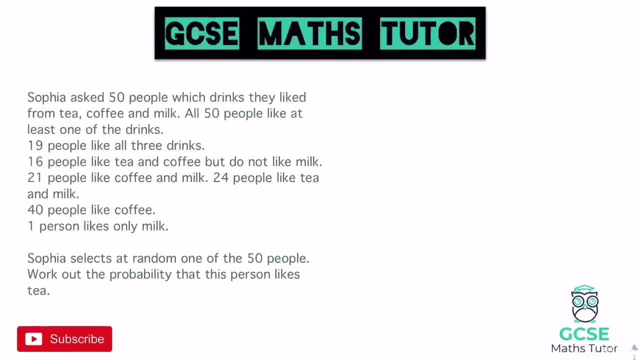 Okay, so the next one. We've got a lot of combinations here. We've got a lot of combinations here. So it says Sophia asked 50 people which drinks they liked best from tea, coffee and milk, and all 50 people that she asked liked at least one of the drinks. 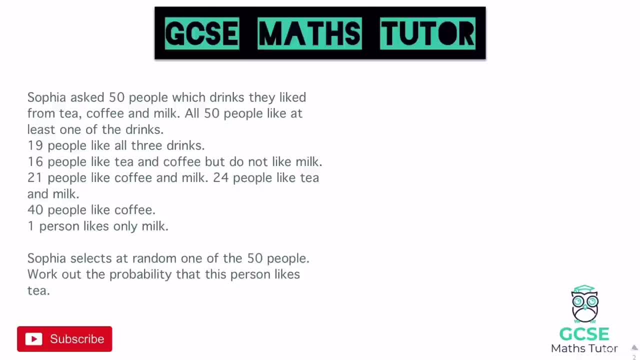 Then it starts to talk about all these different ideas about what drinks people liked and whether they liked all three, whether they liked tea and coffee. So we're going to go through all of them there, but ultimately it says she selects at random one of the 50 people. work out the probability that this person likes tea. 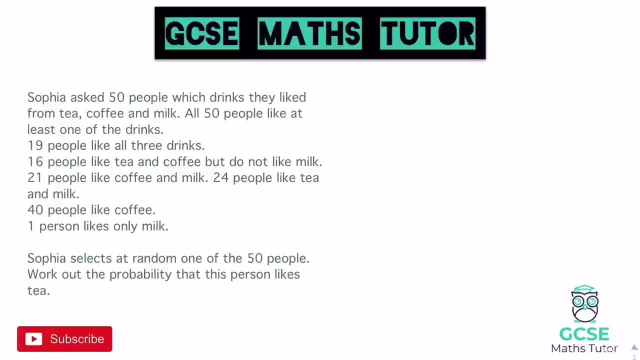 So we need to figure out from all this information how many of the people there liked tea, and it doesn't. It doesn't explicitly tell us how many liked tea. So when we've got these three options like this, the best way for us to organise this is in a Venn diagram, specifically a three-way Venn diagram. 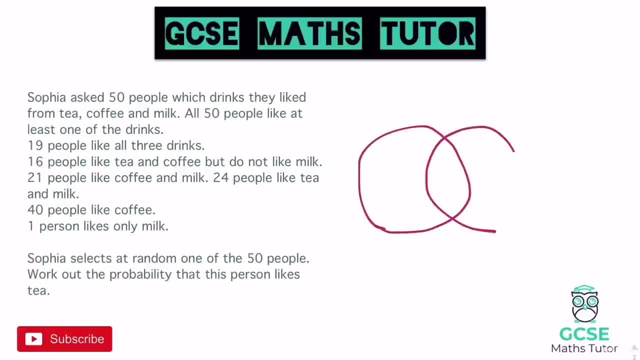 So we need to draw- I'll do this as best as I can- a Venn diagram. It's going to allow us to have three elements in there, and you just need to make sure, with a Venn diagram, you draw your little box around the outside. 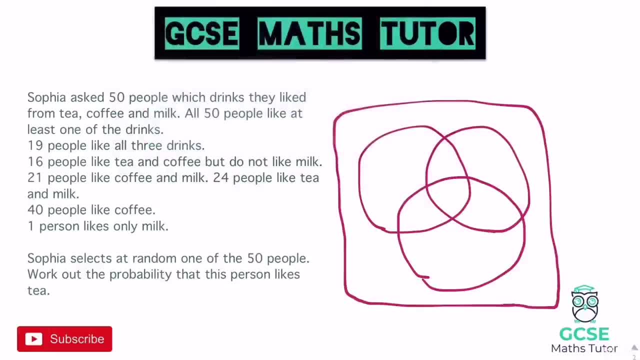 There we go. Now. I want to keep this all nice and neat and tidy, so I'm going to label them. I'm going to call this one the milk, this one the tea, and this one the tea, And this one down here the coffee. 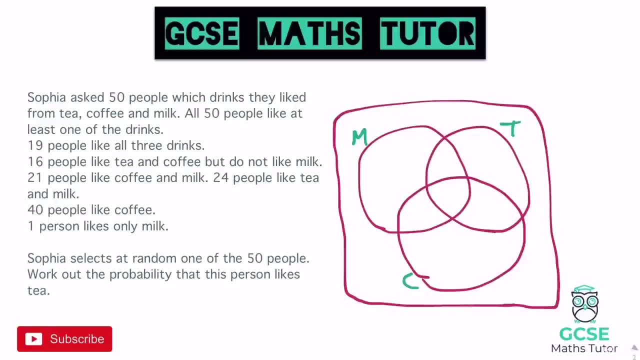 I'm just going to go through the list and just start to tick things in when I know that I've got them there. Now, the first piece of information it tells us- and if we go through this step by step, it says: all 50 people like at least one drink. 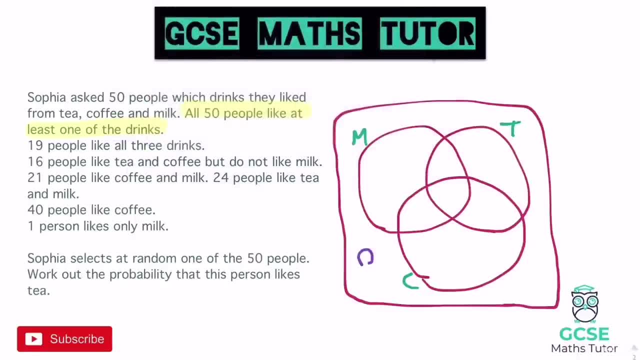 So that means we know that there's going to be nobody in the outside, so zero on the outside. Next thing we've got is 19 people like all three drinks, and that's a key piece of information there, because we can definitely put that in straight away. 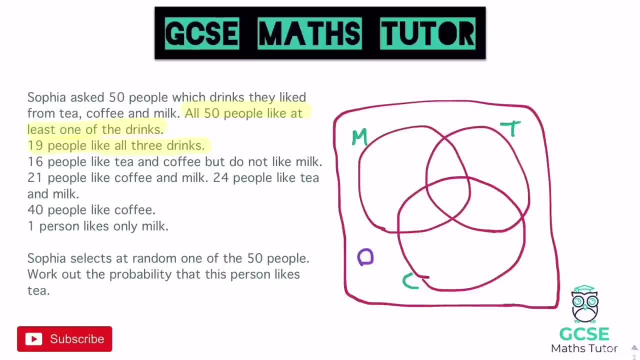 The people that, like the all three, are right, smack bang in the middle there. So we've got 19.. So we've got 19 in the middle, so we've dealt with that one. You can tick them off as you go or highlight them. 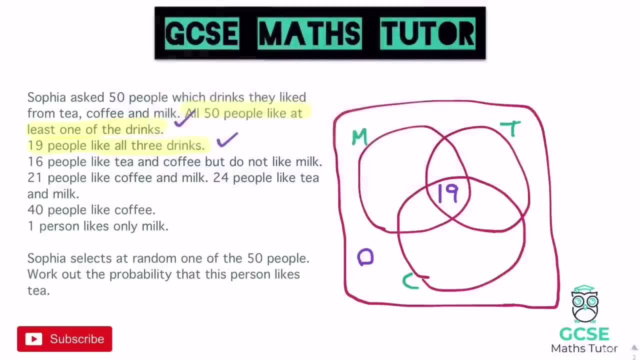 So that next one says it says 16 people. I'm going to sort to a different colour here. It says 16 people like tea and coffee but don't like milk. So the people that like tea and coffee are going to be in the crossover between the tea and the sea circles, but they do not like milk. 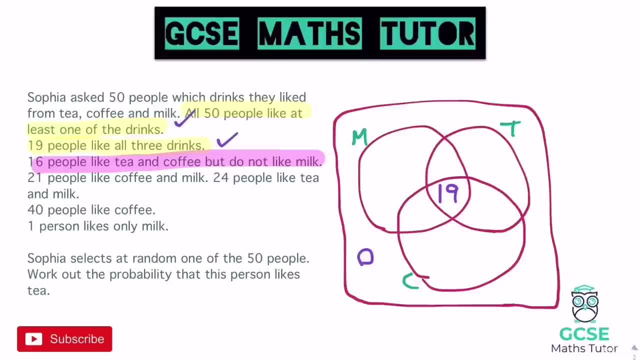 So that's fine, We can put them in there. 16 that like tea and coffee but do not like milk. There we go: Tea and coffee, but don't like milk. It then says 21 people like coffee and milk. 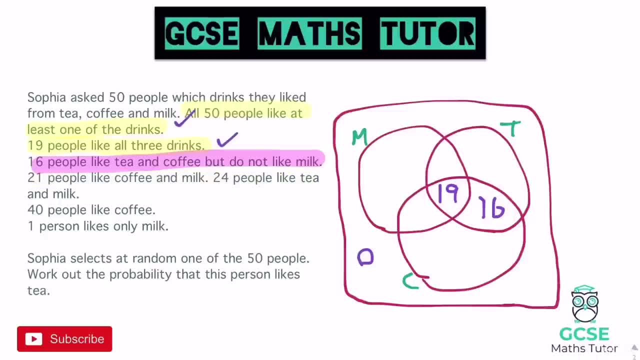 Oh, I'm just going to get rid of that because I've got too many things going in there. I've got 21 people like coffee and milk. So 21 people that like coffee and milk. Well, let's have a look. 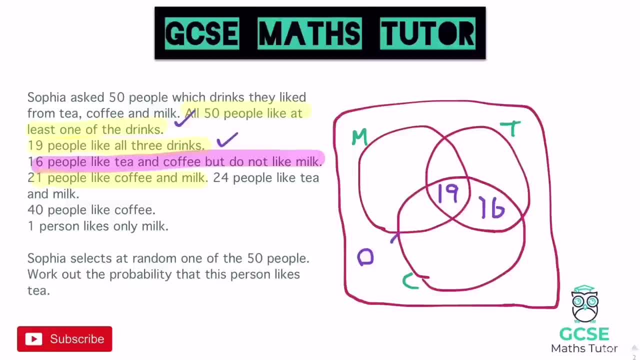 Coffee and milk is this crossover here, but also includes that 19.. It doesn't say: 21 people like coffee and milk but don't like tea. So if 21 people like coffee and milk, we've already got 19 in there. 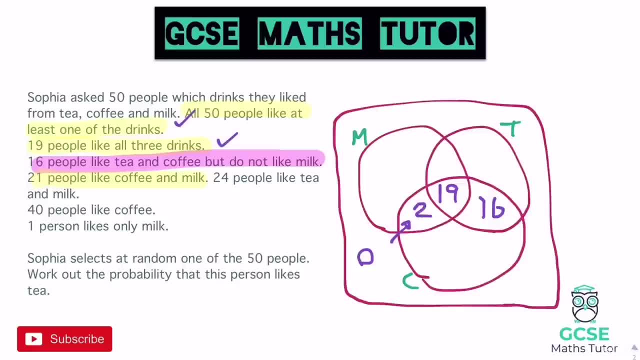 That like coffee and milk. So that's going to be an extra two. that makes that up to 21 there in that little crossover with coffee and milk. 19 of them also like tea, but then 21 in total like coffee and milk. 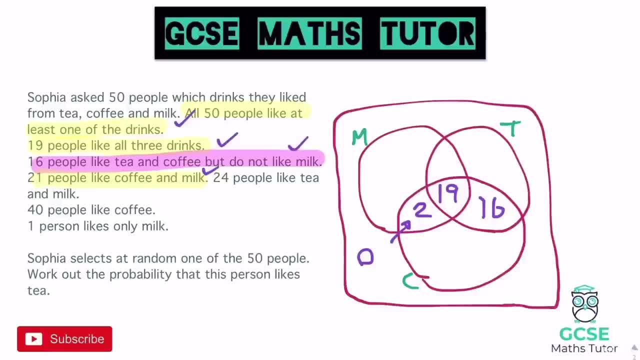 So that's that one dealt with. How many have we done? now? We've done all four of those. There's lots on here. Onto the next one. We've got 24 people like tea and milk. So 24 people like tea and milk. 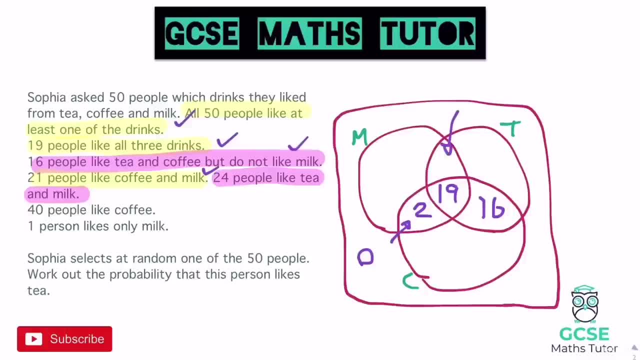 Let's have a look. Well, tea and milk is this one here, but again, it doesn't say that they don't like coffee. So 24 people like tea and milk. 19 are already in there, So that's going to be an additional five people there. 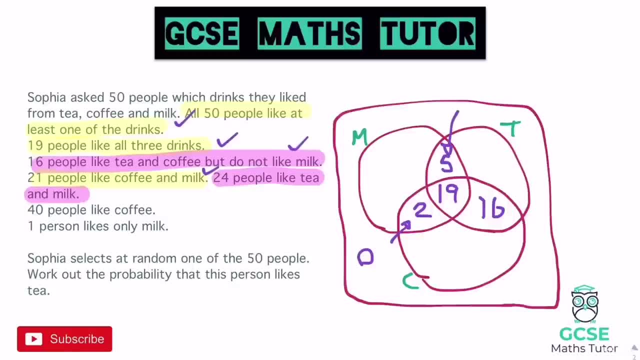 And that makes up 19 and five. That's 24 people in total that like tea and milk. Onto the next one, We've got 40 people that like coffee. We've already got three people in our coffee circle there. We've got the two, we've got the 19 and we've got the 16.. 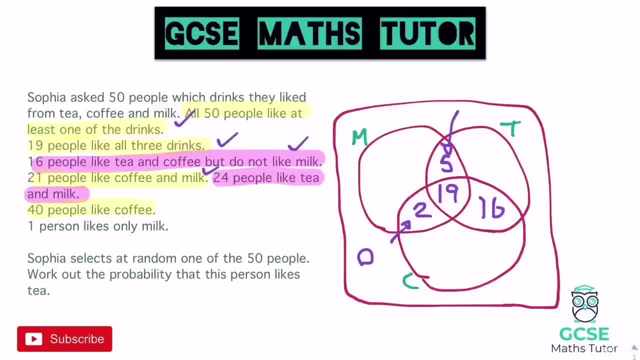 So in total that adds up to. let's have a look: Two plus 19 is 21,. add the 16 is 37 and it says 40 people like coffee. So that's going to be an extra three that make that coffee circle up to 40.. 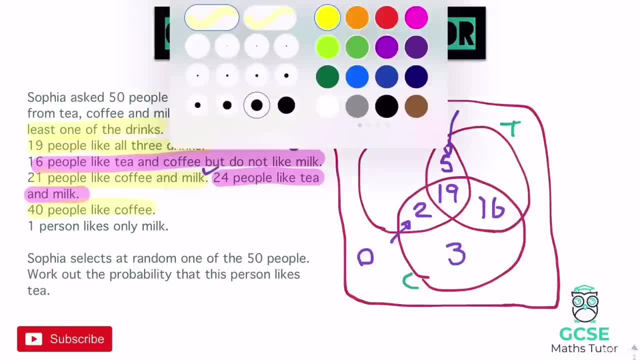 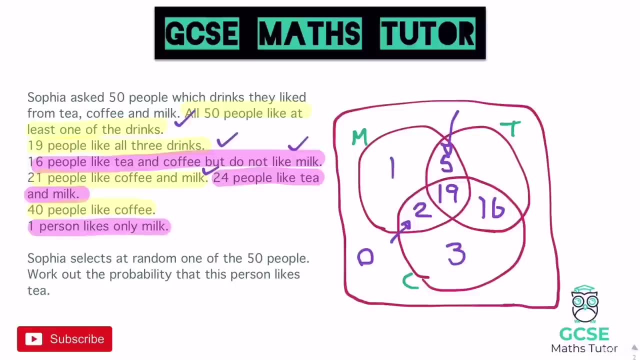 Next one. this one's a nice easy one to finish. We've got one person likes only milk. So in the milk we've got one person and then we're given no more information. But there is this missing number here in the tea. 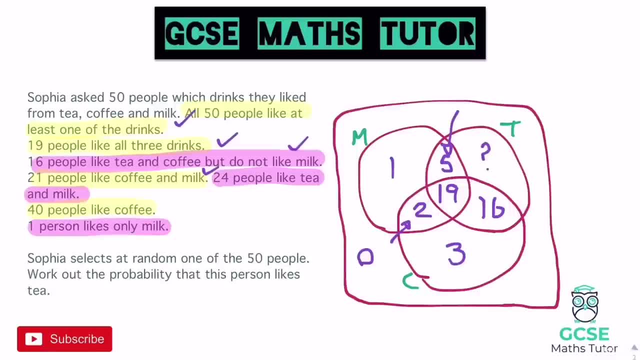 Now just remember it did say in the question that she asked 50 people. So if we add up all the numbers we've got, we've got one plus five plus two plus 19 plus 16 plus three And all of that adds up to make 46.. 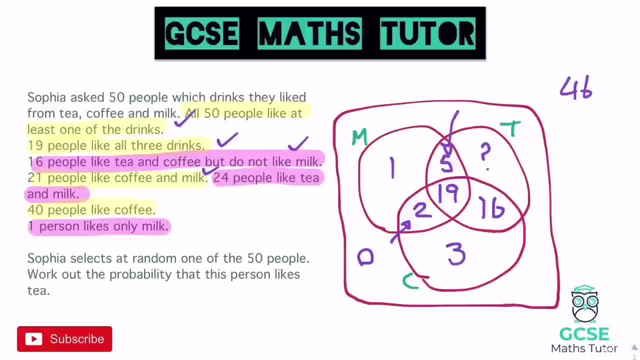 And in total we have to have 50 people in our Venn diagram. So just in the tea one there, that's an additional four people to make sure that we have 50. So we just did 50, take away 46, which left us with those remaining four people. 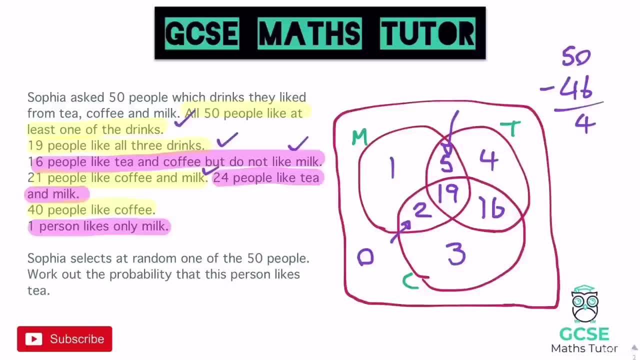 So we filled in our Venn diagram. Now it says: Sophia selects at random one of the 50 people. work out the probability that this person likes tea. Well, that doesn't say just likes tea, it says the probability that they like tea. 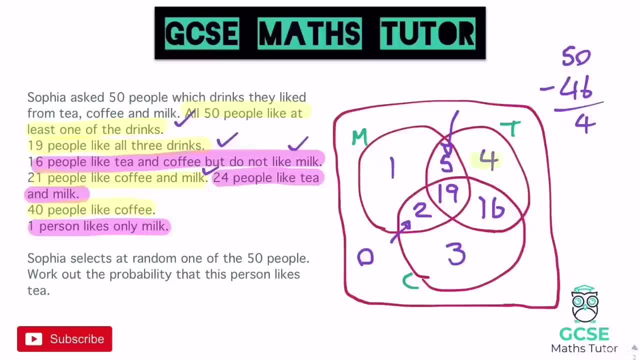 So we've got a few of the numbers here that we can actually consider. We've got the four, the five, the 19 and the 16.. So the prop, If we add them all together, five plus four, is nine. plus the 19 is 28, plus the 16, what? 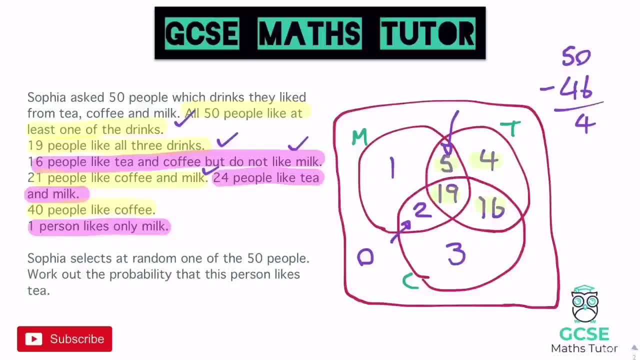 does that give us 19 plus 16. plus five plus four gives us a total of 44 people that like tea. So there's 44 people that like tea out of a total of 50 people. So it's 44 out of 50, 44 of those 50 people like tea and the rest don't like tea. 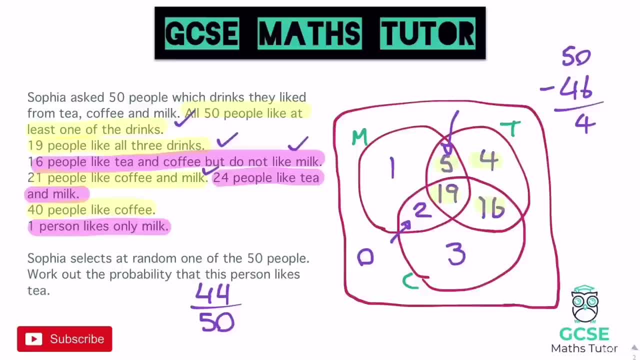 You've got the one person that only likes milk, You've got the two people that like milk and coffee And the three people that only like coffee. So 44 over 50, and you don't need to simplify that. And that's our Venn diagram done. 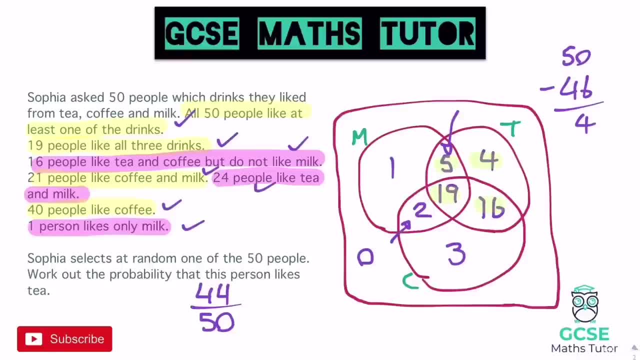 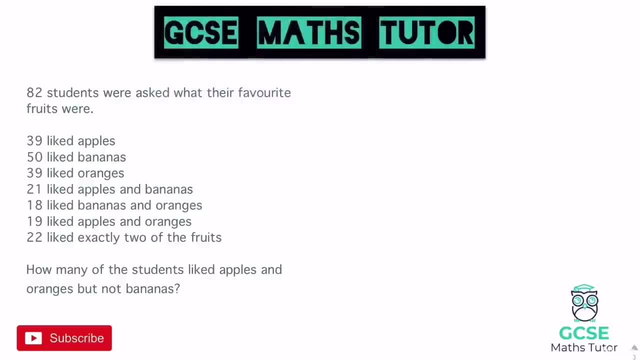 Just make sure you go through and tick them all off as you go, so you haven't missed any. Let's have a look at another one of these. Okay, so this Venn diagram is a little bit more complicated. It says: 82 students were asked what their favourite fruits were: 39 like apples, 50. 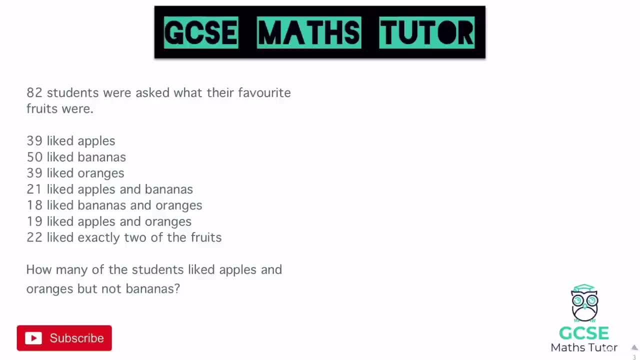 like bananas, 39 for oranges, 21 like apple and bananas, 18 like bananas and oranges, And we've got some more information there, but the one we're looking for is the amount of people that like all of them, And this doesn't actually tell us the amount of people that like all of them. 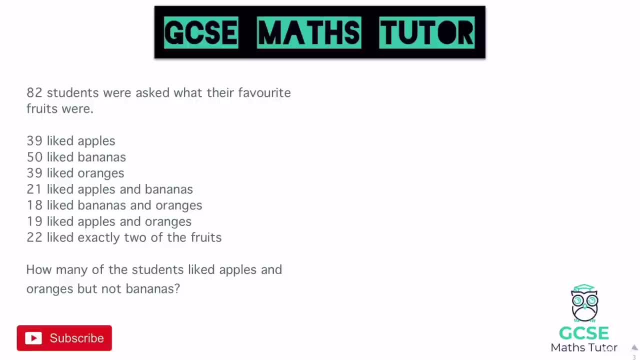 So we're going to have to take a little bit of a different approach here. but just say how many of the students like apples and oranges but not bananas. So we're going to look for those people in a sec. Now, if I draw a little Venn diagram for this one, again I need a little bit more space. 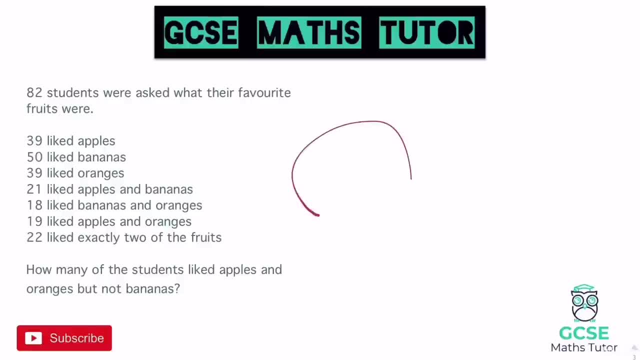 and might actually make that a little bit bigger. Let's make this one a bit bigger. Okay, so we've got our Venn diagram again. nice little box on the outside, and let's have a look at what needs to go in here. 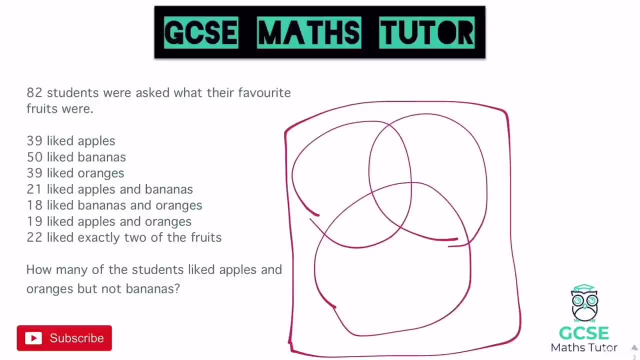 So 82 students were asked what their favourite fruits were, So we know that 82 people are going to have to go into our Venn diagram Now. it says that we've got lots of different bits of information, haven't we here? So let's just label it up so we can keep it nice and clear. apples, bananas and oranges. 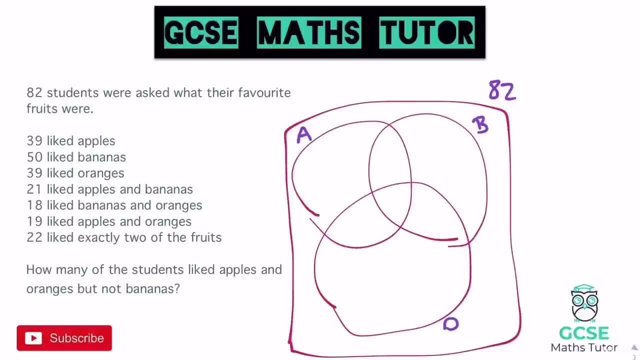 down here, Not to mistake that for zero people there, that's oranges. Now we don't know how many people are in the middle, so we're going to apply a little bit of algebra here. I'm going to say, okay, well, there is an amount of people in the middle and we'll call that. 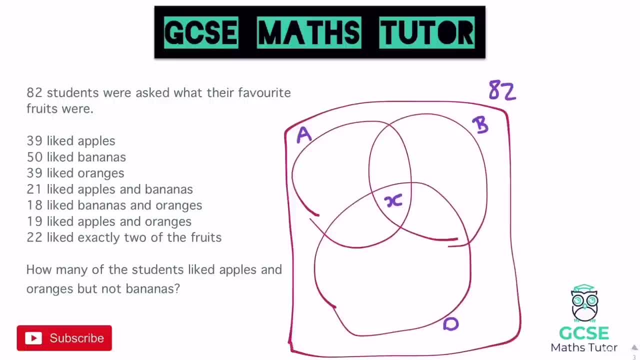 X. Okay, So I'm just going to start to have a look at some of the other bits of information. I'm going to disregard the apples, bananas and oranges bit to start with, but what I am going to do is just label that up here, just so I remember. 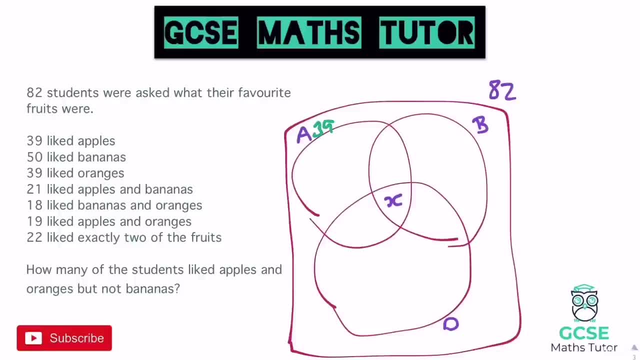 So apples is 39, so we know 39 in total in that circle. Bananas is 50, so we know there's a total of 50 going into that circle. And oranges is 39, so we know there's a total of 39 going into the oranges there. 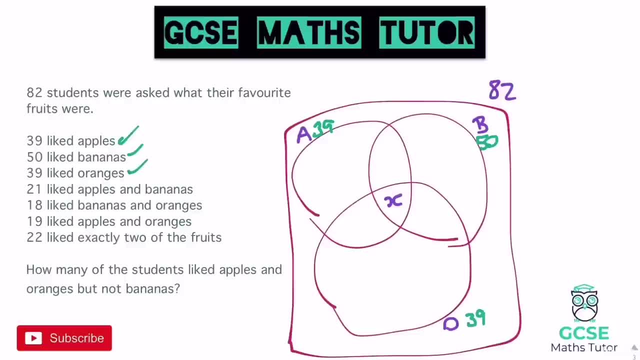 Okay, So I'm going to tick those all off. I've drawn them on my Venn diagram. I'll remember that later. Now it says: there we go. 21 liked apples and bananas. So 21 like apples and bananas. 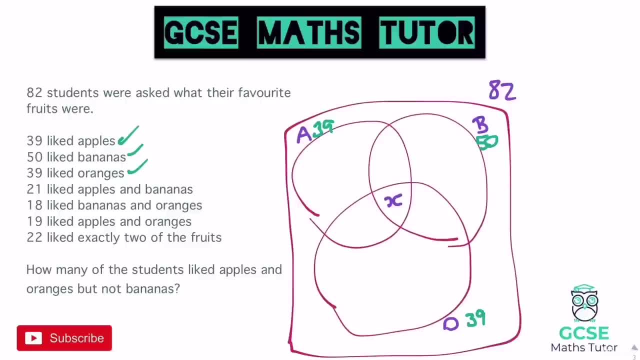 So that is going to be 21 in total, including that crossover. that's going in these two just here where the apples and bananas crossover. So if I knew what the middle number was there, I'd do 21,. I'd take away the value of X in. 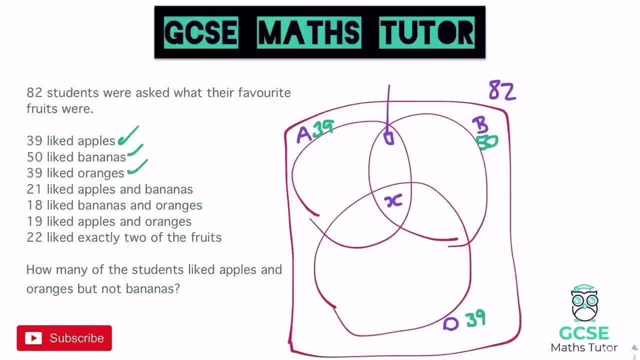 the middle. but I can't. I don't actually know what X is, so I'm just going to write in here: that's 21 minus X for that one. Okay, So that's that one done for the moment in terms of algebra. 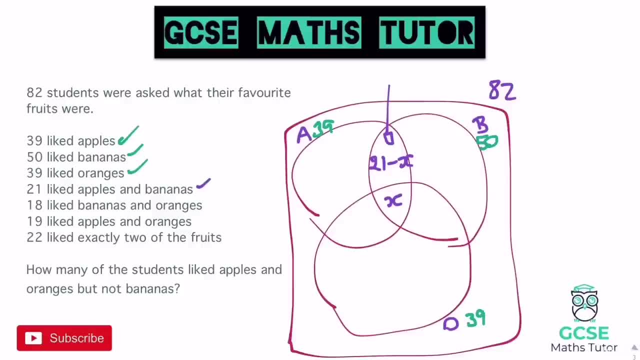 Then we've got 18 that like bananas and oranges. So bananas and oranges is just here, but again we don't know what that middle one is there. It doesn't say that they're like bananas and oranges but not apples. So that's going to be 18, take away the middle number, which again is X, 18 minus X. 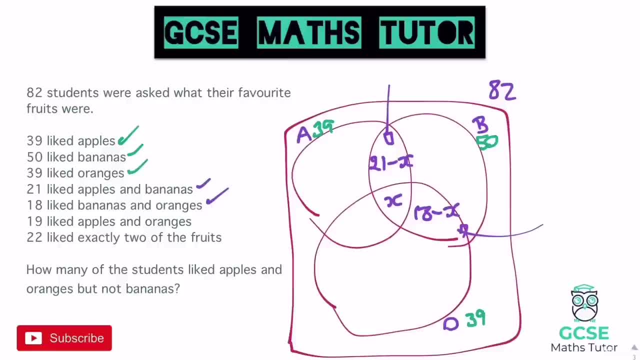 Onto that last one. we've done this one now. So 19 liked apples and oranges, And again that's this one here: apples and oranges. but again we don't know the middle number, So we'll call that 19 minus X. 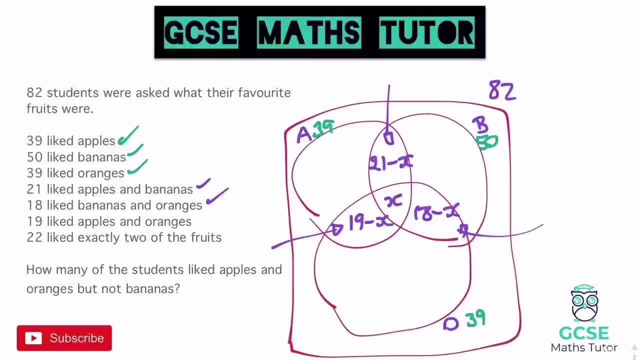 There we go. So there's our bits of algebra. let's tick that off, Okay? So it says 22 like exactly two of the fruits. Now, the people that liked exactly two of the fruits are the first one we did: 21 minus. 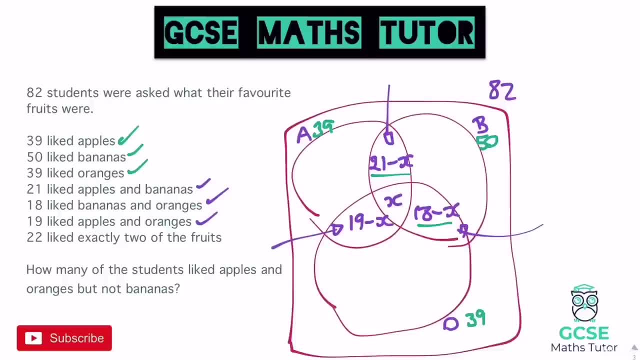 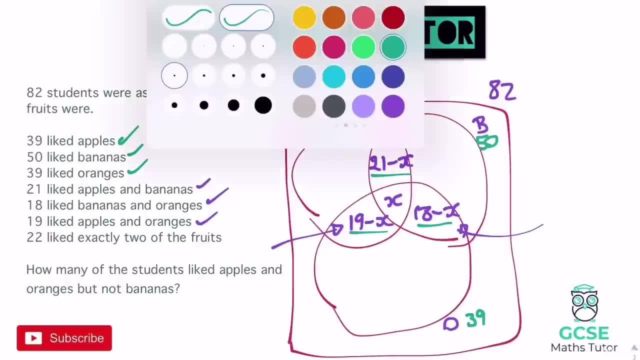 X that like apples and bananas. We've got 18 minus X that like bananas and oranges, and we've got 19 minus X that like apples and oranges. So what we can actually do is we can create a bit of an equation here. 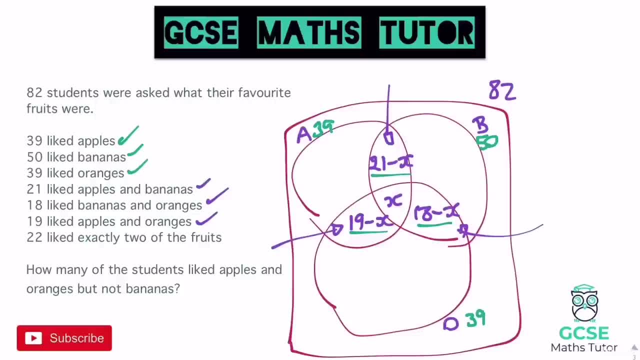 Now if we add those all together, that has to equal 22,. because it says 22 here liked exactly two of the fruits. So if we add them all up, let's have a look, Let's just add them all up, So we've got 21 minus X, we've got 19 minus X and we've got 18 minus X. and if we add, 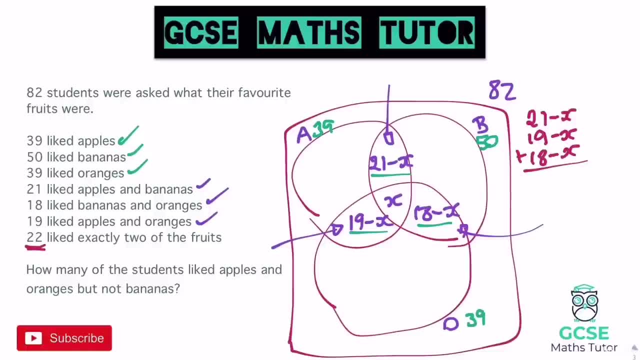 them all together, let's see what we get. So 18 plus 19 plus 21 gives us a total of 58, so we have 58 minus three Xs. so minus three X. So actually we can create a bit of an equation here. 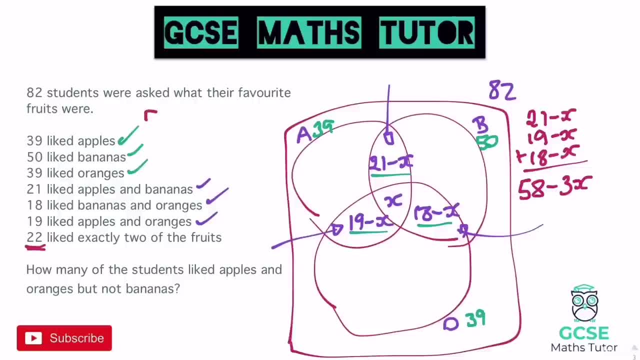 I'm running out of space a little bit, so I'm going to do it over here. but we have this equation: We've got 58 minus three Xs- Okay, We've got 58 minus three Xs- and it says it has to equal 22 people. 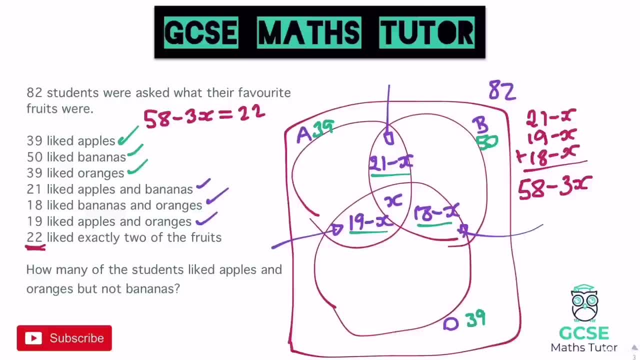 So actually we can just go about solving this now. So actually what I can do, and we can rearrange it if we like, but I'm just going to minus 58 from both sides. So 22 minus 58 gives us negative 36.. 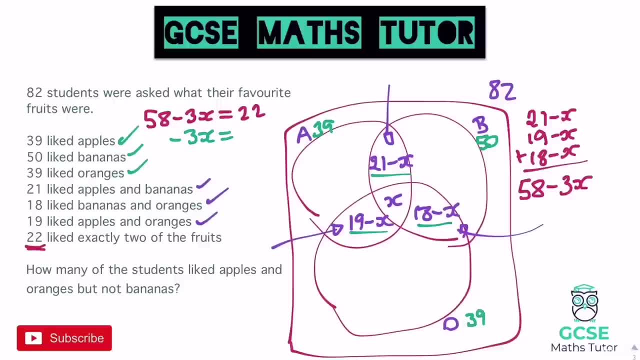 So we have negative three. X equals negative 36, and if we do negative 36 and divide it by negative three, that gives us a value of X which is 12.. So we know that X- that one in the middle- now has to be 12.. 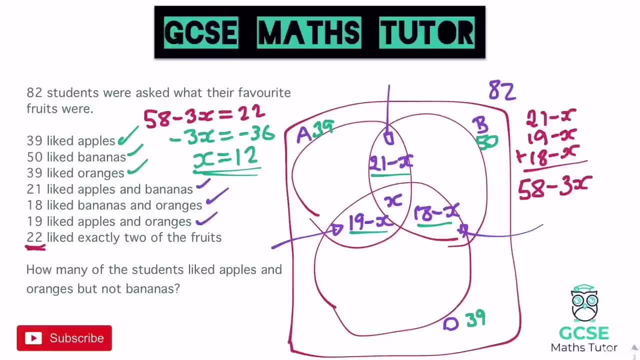 So, actually, what we can do, we can start to get rid of some of these numbers and actually, sorry, get rid of some of these Xs and replace them with numbers. So if I get rid of the X in the middle and we'll replace that with the 12, because we 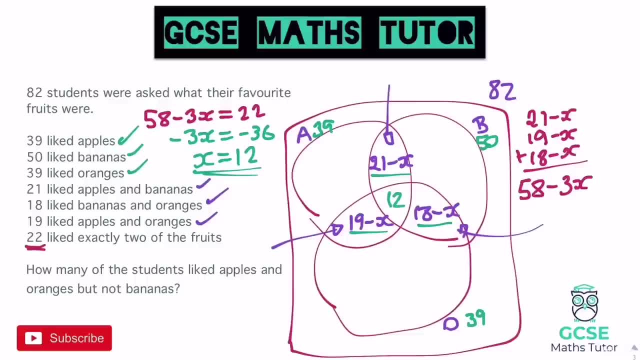 now know that 12 is in the middle. we can then do 21 minus X above that, which leaves us with nine. So we can get rid of 21 minus X. Oh dear, got rid of the whole circle there. We can get rid of 21 minus X and we can just put 21 minus 12, which is nine. 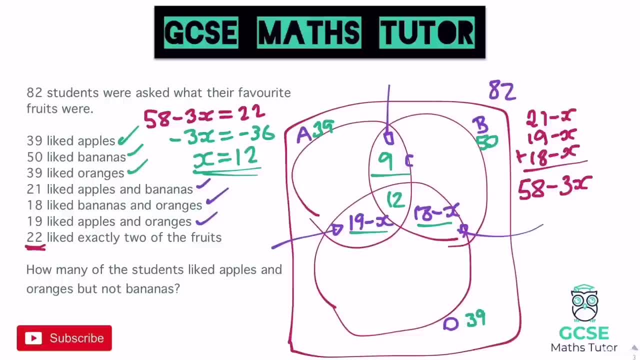 So there's nine going in there, We can get rid of 19 minus X. 19 minus 12 leave us with seven, so we can get rid of that, And we just got seven in there. And then we've got 18 minus X on the right there, and 18 minus 12 leaves us with six. 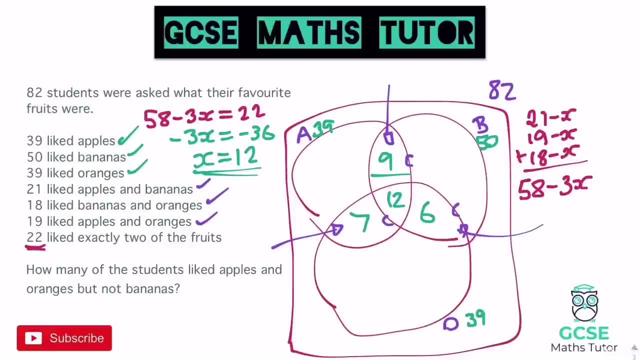 So we can have six in there. There we go, Six. We might be able to answer the question from here, but let's go ahead and fill in the rest of the Venn diagram as well. So we know that in A there's 39 in total and we've got nine, 12, and seven. that's already. 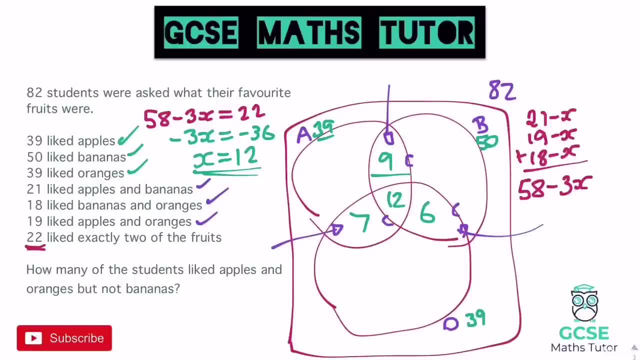 in there. So we've got nine plus 12 plus six is 28.. So we need an extra 11 in the apples there to make it up to 39.. Moving on to the bananas, Again we've got nine, 12, and six, and nine plus 12 plus six is 27.. 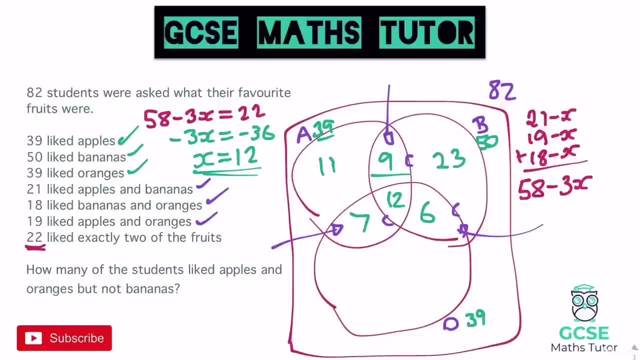 We want to get to 50, so that's an extra 23.. And then in the bottom one we've got seven plus 12 plus six, adding up to 25.. We need 39 in there down the bottom, So that's going to be an additional 14.. 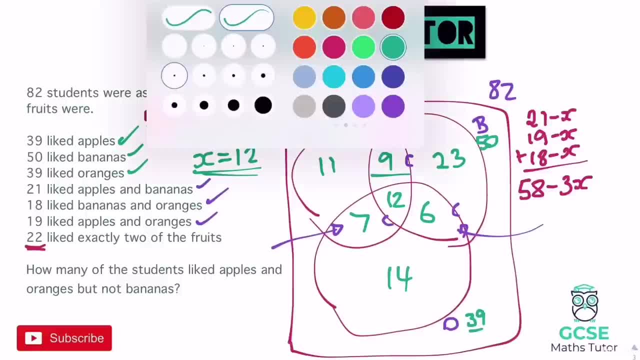 Right, there we go. So that's our Venn diagram filled in Now. the question said not to finish what it was actually, not to forget what it was. but the question said not to finish what it was actually, not to forget what it was. 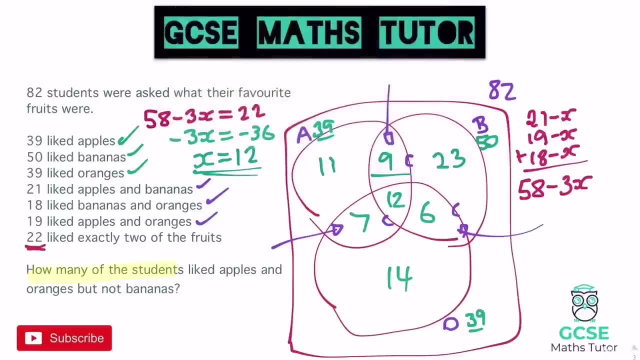 actually, But to forget what it was actually asking us here. it said how many of the students like apples and oranges but not bananas. Now the ones that like apples and oranges but not bananas are here. Let's highlight it: These ones here like apples and oranges but they don't like bananas. 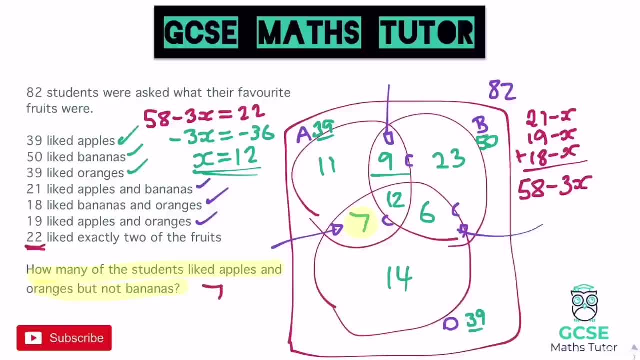 So we've got seven people there. So we've got a total of seven people out of the 82 people in total, And that will be our final answer. There we go. So you can apply this to a Venn diagram. that's not a triple Venn diagram where you've just 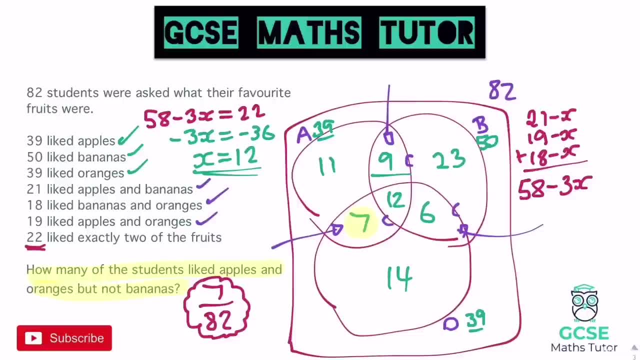 got a normal two, Two circle Venn diagram as well, But when it doesn't give you that crossover number there, you do have to think about how you can apply algebra to this. So that's quite a complicated one there, but just a little example of how you can approach. 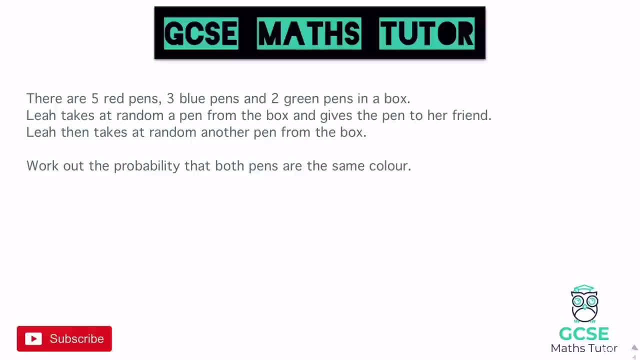 some of these harder Venn diagram questions. Okay, and some probability here. It says there are five red pens, three blue pens and two green pens in a box. Leah takes at random a pen from the box and gives the pen to a friend. 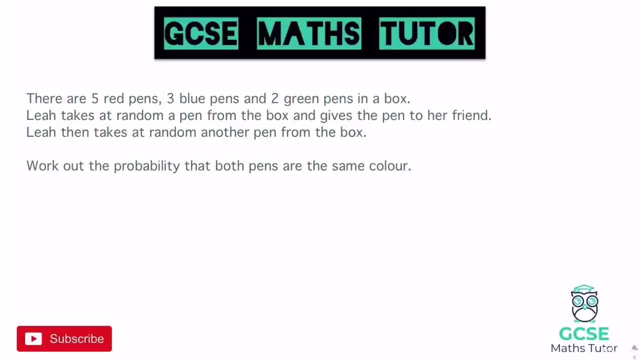 Leah then takes at random another pen from the box to work out the probability that both pens are the same colour. So we can do this using a probability tree. So we can do this using a probability tree, But there are three things. So I'm going to have to have three branches here and it can get quite messy. 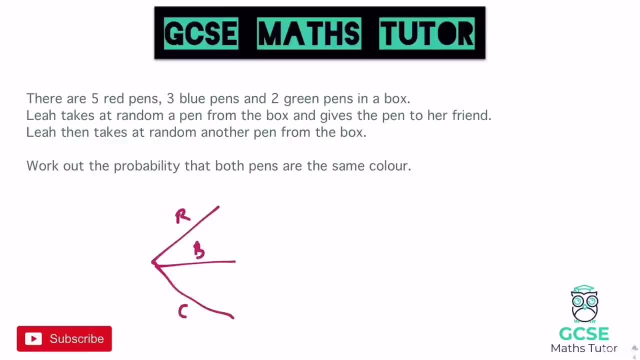 So we've got red, we've got blue and we've got green. Now in total there we've got five red pens, three blue pens and two green pens and in total that adds up to ten pens. So this is going to be all out of ten pens here. 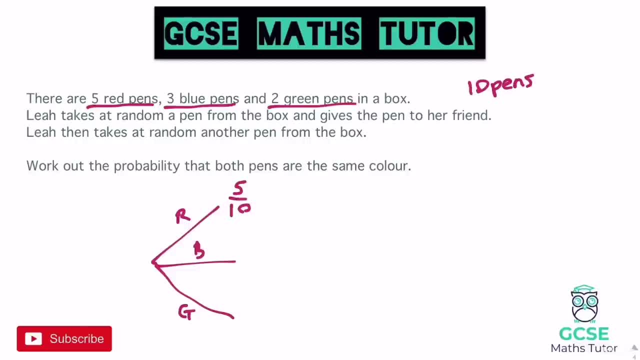 So the probability of getting a red is five out of ten, The probability of getting a blue is three out of ten And the probability of getting a green is two out of ten. Now it's up to you. We can do all three branches coming off these, if you want, for that second picket. so she 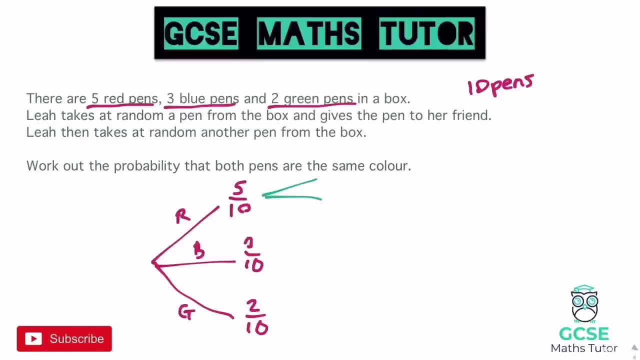 doesn't replace it. So off each branch you've got red, blue green, red blue green and red blue green for the bottom. But really we're only really concerned here about the same colour. So I want to know what's the probability of red on the second picket if we take a red? 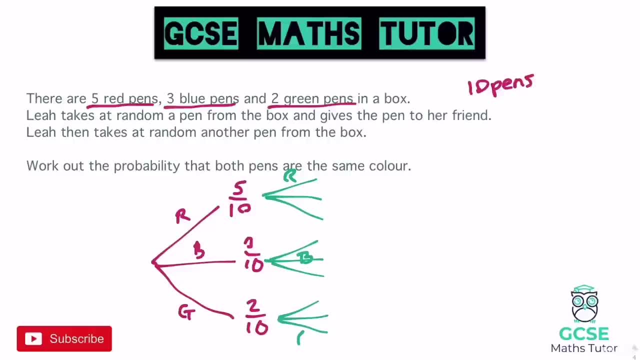 What's the probability of blue here, if we take a blue, And what's the probability of green down here if we take a green? Now, if we think about this, there are five red pens in the box. So if we were to take another red pen, that would reduce down to four, so there would 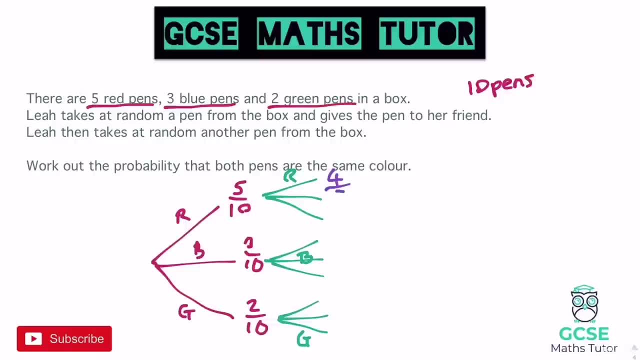 only be four red pens left, and now there'd only be nine in the box, So we don't need to fill in every branch on the tree here. We could do. we've still got three out of nine for blue and we'd still have two out. 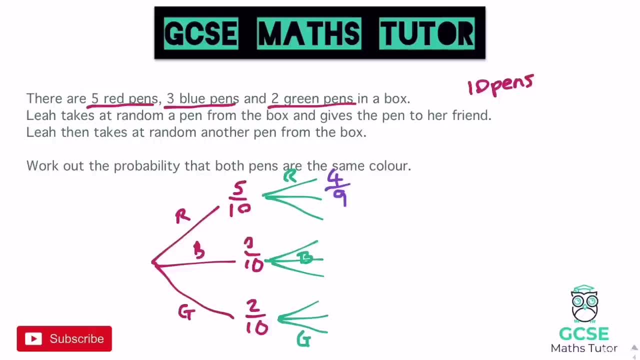 of nine there for green, but I only really care about the probability of getting another red at this point. Moving on to the blue branch, so down here we have three blue pens in the box, So if we take one out, we've now only got two blue pens, and again, that's going to be out. 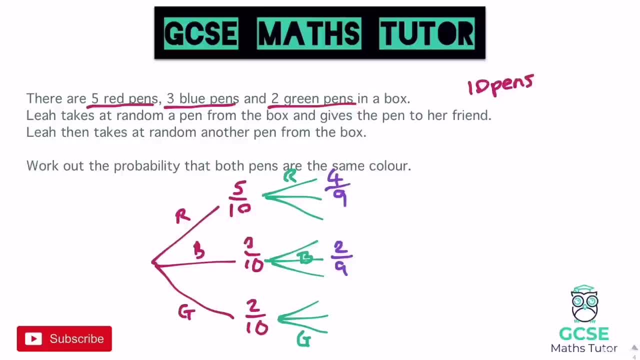 of nine. So that's the probability of getting a blue. if we took a blue on the first pick, And then the final scenario down here, if we took a green on the first pick, we'd only have one green left and again there'd only be nine in the box. so that'd be one out of. 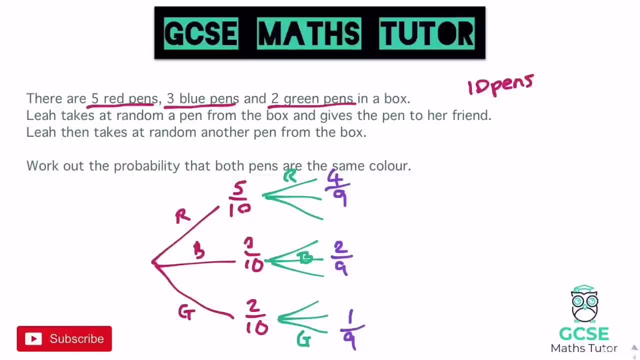 nine. So there's the probability of getting this second colour when it's the same. So, just like normal probability trees, we just need to work out these three probabilities here. So for the first one we'd do five over ten multiplied by four over nine, which is nice. 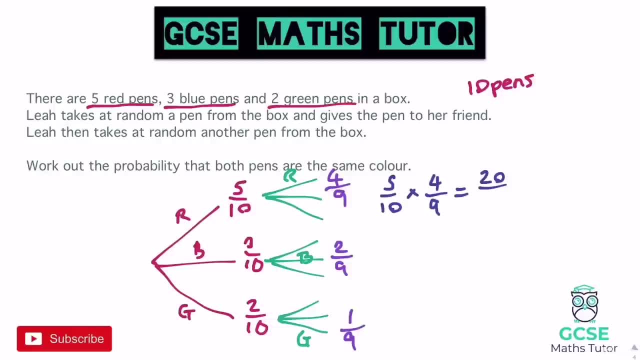 and easy for us to do. Times. the top is 20, times the bottom is 90. Into the middle, In fellow four, we've got over ten multiplied by two over nine, and again that's going to be over 90, but with three times two on the top, which is six and a ninety. 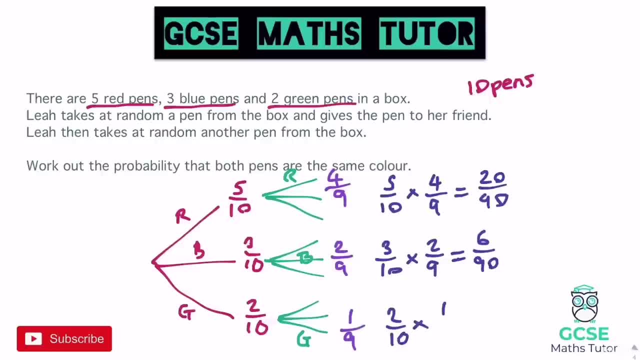 anh, bottom again. And then the final one. we've got two over ten multiplied by one over nine, and one times two is two and again ninety on the bottom. So there's our three probabilities. We've got the probability of getting red- red of 20 over 90, blue- blue would be six over. 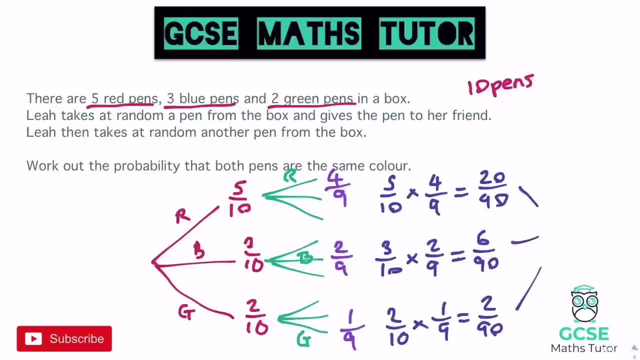 90, and green green would be two over 90.. all we have to do is add them all up. so add all of these together to get our total probability. let's just put some plus signs here and 20 on the top. plus 6 is 26, plus 2 is 28, so our final. 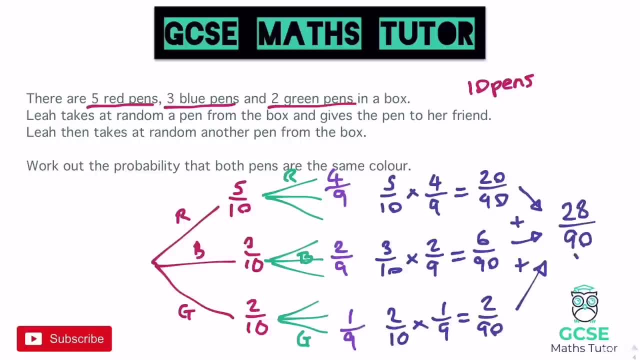 probability there would be 28 out of 90, and again, you don't need to simplify that. so that'll be your final probability there. you go a little bit of a trick there when you are constructing these trees. if you only need certain branches, then you can just kind of ignore the others, but just be very 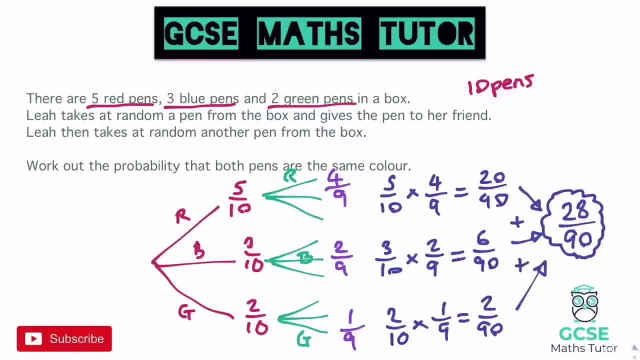 careful what the question is asking for, because it could have asked us for different colours there. just on a side note. if it did ask us for different colours, that would have obviously been the other six branches, but you can also save your time just working out the three that we don't need. 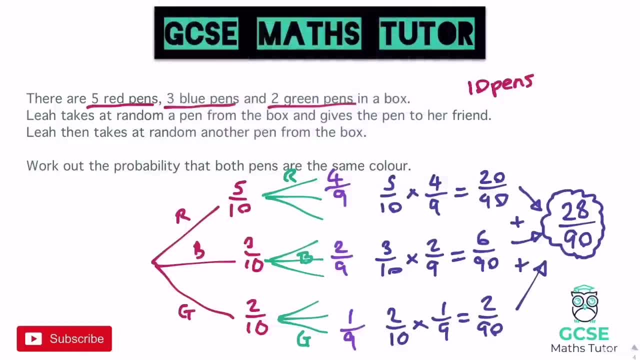 and then we could take that numerator there, 28 away from 90, so the probability of different colours would be 62 over 90. what's left over there? different colours? okay, that would be only, though, if it said different colours, and this particular question did say the same colours, so just be. 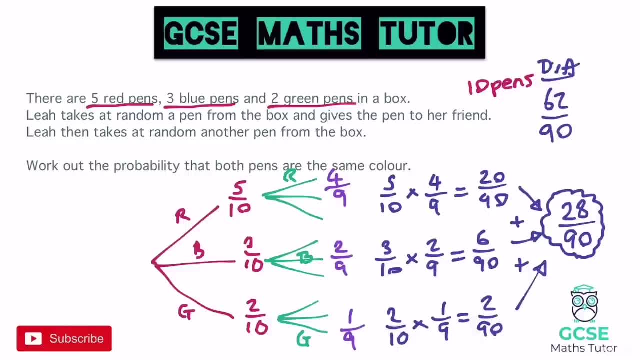 careful, but you could save yourself a bit of time. rather than working out all six, you could just work out these three, and then you could just save yourself a bit of time, and then you could work out all six. you could just work out these three, and then you could save yourself a bit of time. 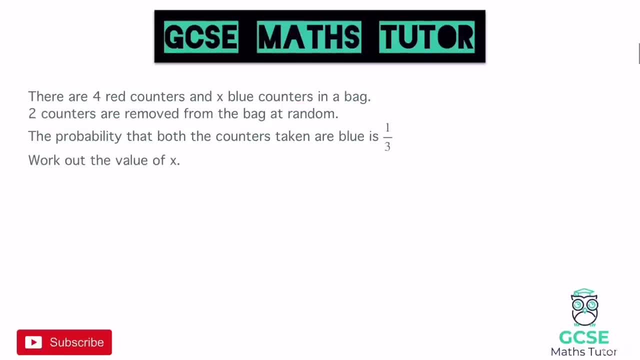 take it away from 90 for your numerator. onto the final question here on probability trees. it says there are four red counters and x blue counters in a bag. two counters are removed from the bag and the probability that both the counters are taken is blue is one third. work out the value of x. 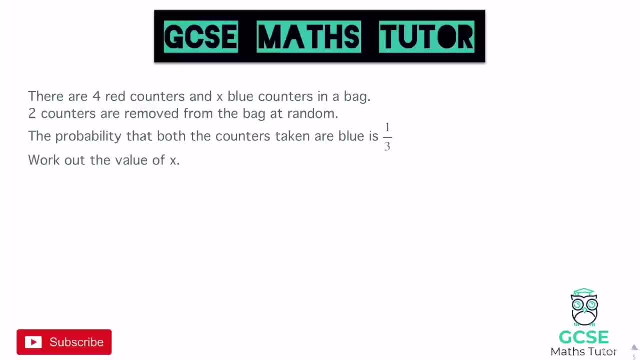 now the tree here isn't so nasty to construct, but we have got some algebra going on in the tree now. what it says is there are four red and x blue. now so for the total amount of counters here. we don't actually know what the total is, but we could write it in terms of algebra. 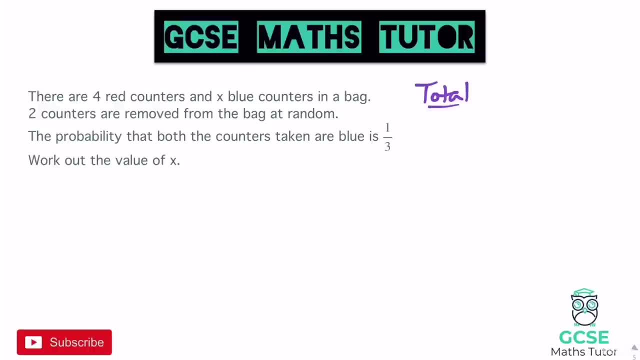 if we knew the amount of blues, we just add it to the amount of reds so we could say: it's x plus four is our total and that's going to be our denominator on our tree here. so if we just construct two branches for our tree, we've got red and we've got blue and the probability for red. 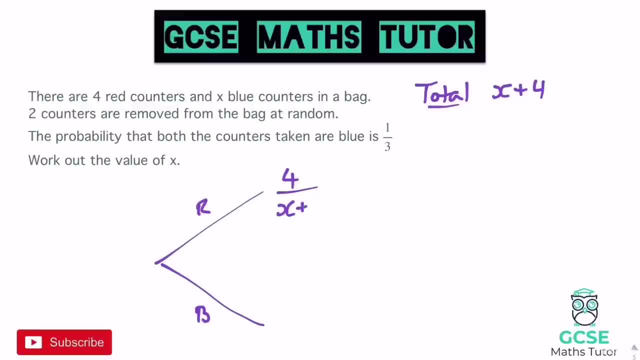 there is going to be four out of x plus four and the probability for blue is going to be x over x plus four. now again, really, the only proper part of the tree here we're actually considered, um, you know, we want to consider is the probability of x plus four and the probability of x plus four. 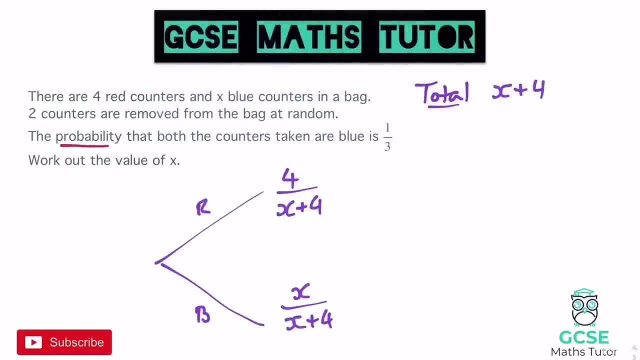 is the probability for both of them being blue, because it says the probability that the both counters are blue is a third. so i don't really need to do the whole tree here. i just need to have a look at this probability down here. and that would be if i took a blue on the second pick. 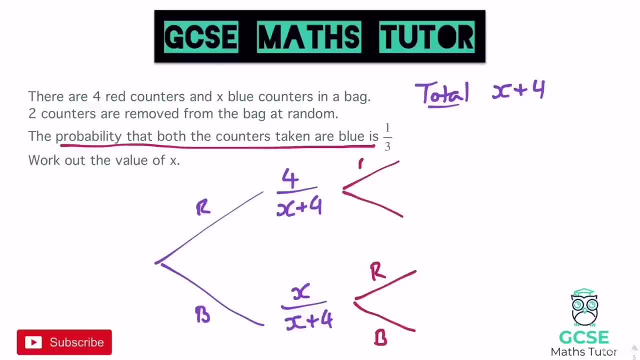 but again, i'm actually just going to go and construct all the branches here so that we can just discuss them, but we only actually need the one at the bottom now. if we took a red, that would reduce our amount of reds down to three, because there are four reds in there at the moment. 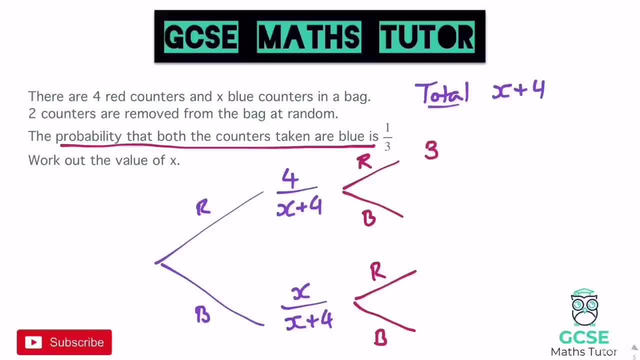 so if i imagine that we've taken a red out, we would only have three and that would no longer be over x plus four because one of them's gone. so it'll be over x plus three, reducing that denominator by one. again onto the blue branch if we take um one of the reds out. 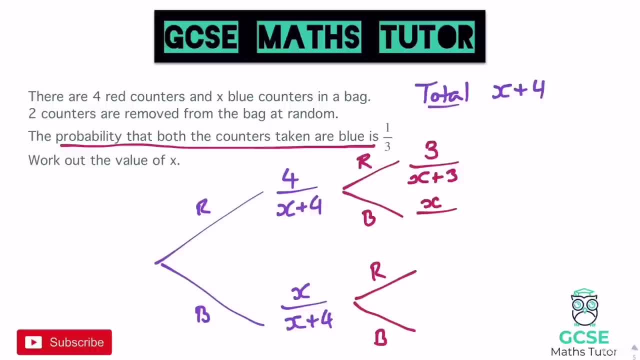 obviously none of the blues have actually gone, so we've still got x blues, but that is going to be over x plus three. again, all the denominators are the same onto the bottom half of the tree. if we took a blue out on this bottom half, the amount of reds would be the same, so we would have four. 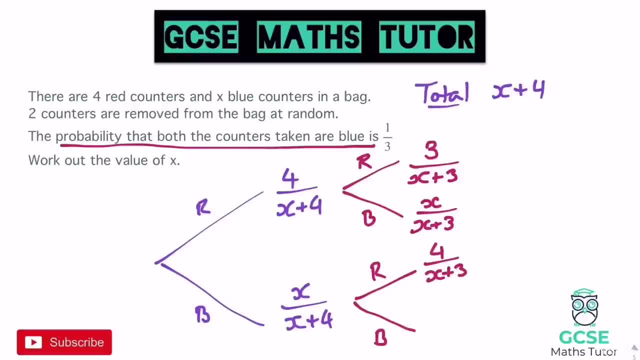 still over x plus three, because we've lost one on the bottom, and the one that we're really concerned about is the bottom one, which is if we took a blue out. we don't know how many blues there are, so we'd have to just say, okay, well, that'd be x minus one, counter over x plus four, and that's how we can. 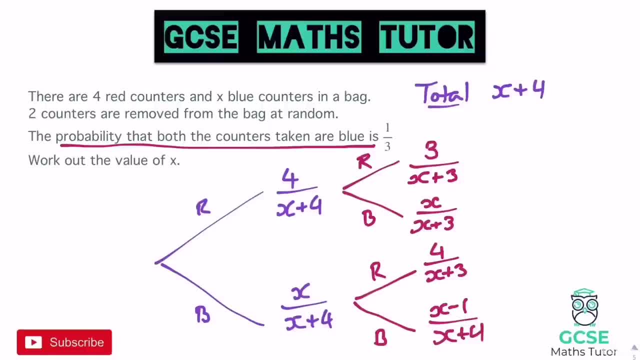 construct a probability tree using using algebra here. now what it says is: it says that those probabilities down here, so the probability of getting a blue and then getting another blue, is one third. so when you times these fractions together, it says they're going to equal a third. 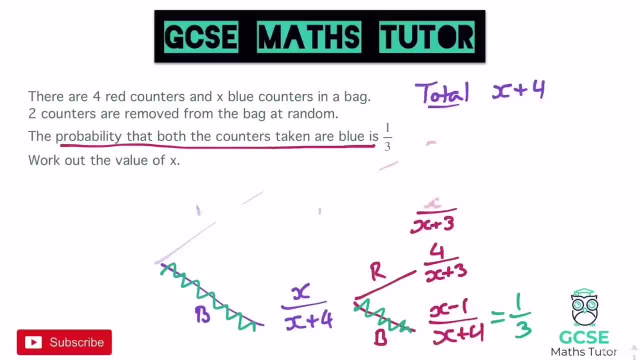 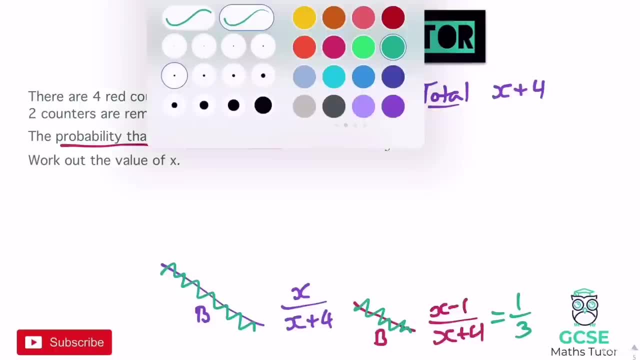 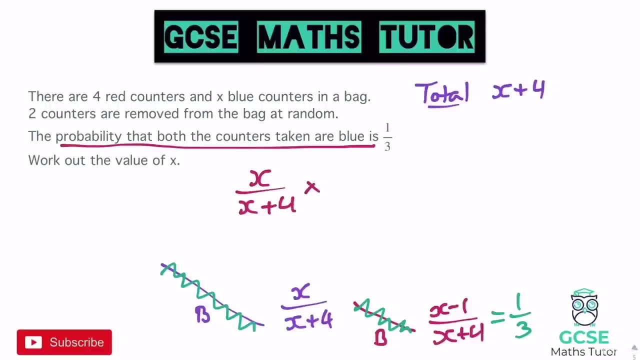 so if i try and get rid of a lot of this tree here, because we're only really crucial, we're going to add in a number of three, so for that we just say we've included the next one and the next one, and so after that sprinkle the code for ourWORL effic clich. so 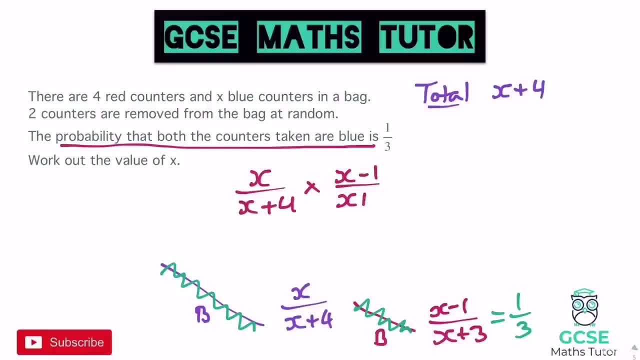 explain some how you done that. so iHop on IHop on c chopped. that came out okay that all of that equals 1. 3rd. Obviously I've got a limited space here, so I'm going to get rid of that tree now that we've corrected that denominator and we've just got to actually work out all of. 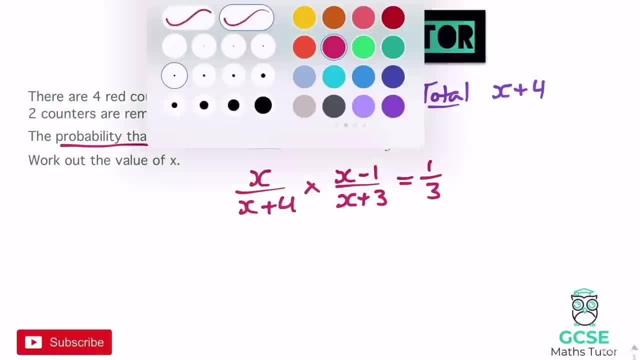 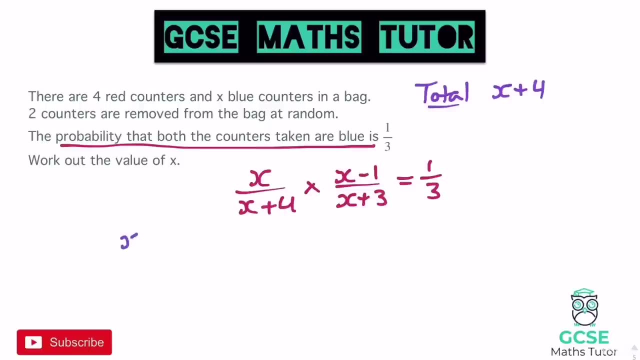 this algebra here and we've got a bit of an equation. So if we go about working this out now, if we multiply these fractions together, multiplying the numerators x times x minus 1, gives us x squared minus x, and if we multiply the bottoms there we have a double bracket to work out. 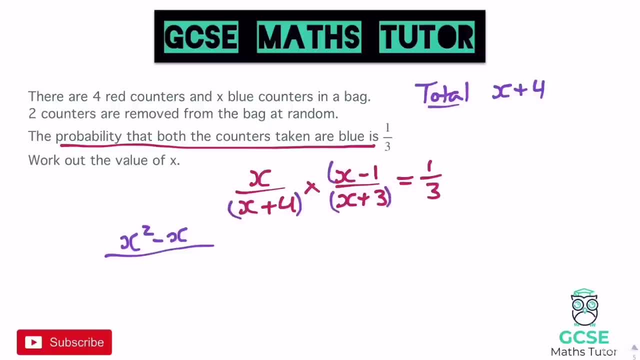 Okay, so you can imagine these are in a double bracket. that first one was like a little single bracket: x times x minus 1.. So if we multiply out the double bracket here, we get x squared plus 4x plus 3x, which is plus 7x, and 4 times 3 is 12, so plus 12, and it says that that equals 1. 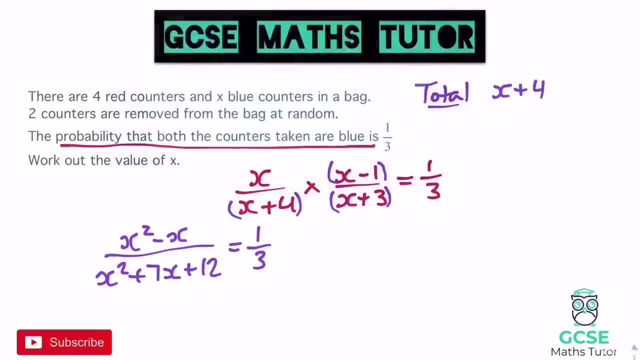 third. Okay, so from here we've got to cross multiply to get rid of these two denominators. so I'm going to times the denominator over here up to the 1 and the 3 up to the other side there, so timesing both sides by 3 and timesing both sides by this quadratic on the bottom, the x. 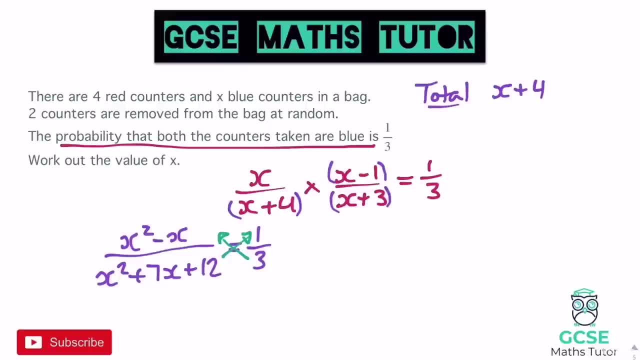 squared plus 3.. So I'm going to times the denominator over here up to the 1 and the 3 up to the 7x plus 12.. So if we do that, I'll write this out as a like a step you can see. to start with, we'd have 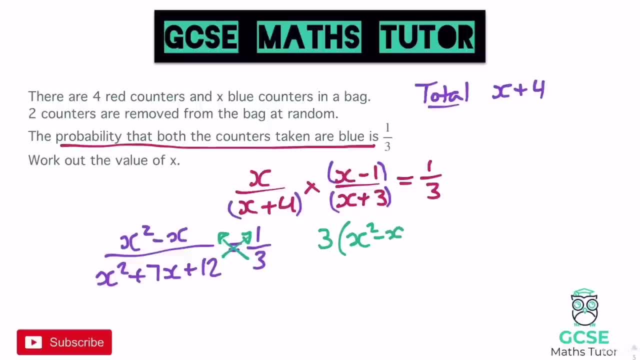 three lots of x squared minus x equals one lot of- so I won't write this in a bracket- but one lot of x squared plus 7x plus 12, and now we can actually go about solving this. So obviously we need to expand this bracket out to start with. so times these both by 3 and we get 3x squared minus 3x. 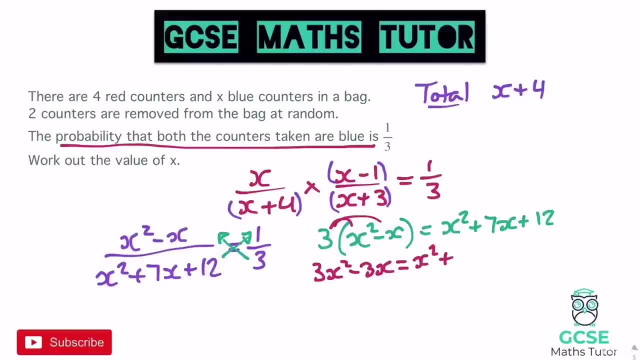 equals x squared plus 7x plus 12.. Now, just like with all quadratics, we may need to make this equal zero. so I'm going to move everything to the left hand side, so I'm going to subtract all three of these pieces. I'm going to subtract x squared, which would leave us with 2x squared when we 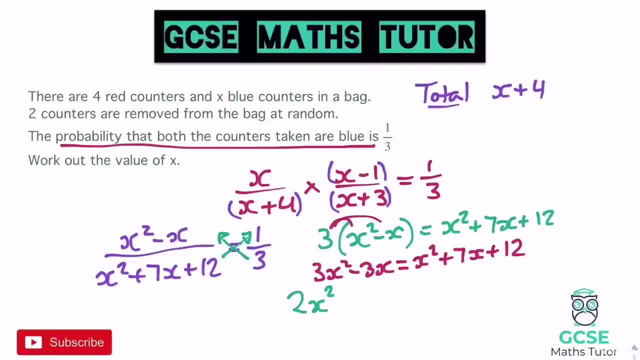 take x squared from both sides, I'm going to take away 7x from both sides, which would leave us with negative 10x over here, and I'm going to take away 12 from both sides. we haven't got a number on the left, so it's just going to be: take, take away 12 there, and now it equals zero, So I'm going to take. 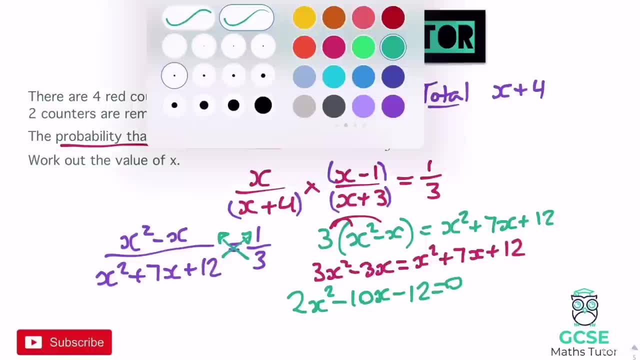 away 12 from both sides. we haven't got a number on the left side, so I'm going to take away 12 from Now we can actually go about solving this. so we can either factorise or use the quadratic formula. this one, I think, does actually factorise, but we can simplify it first. we can divide everything by: 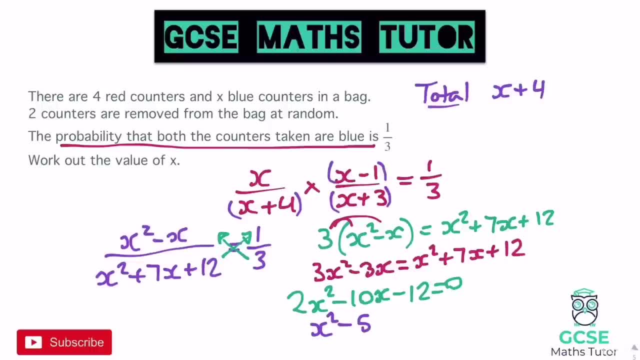 2. so if we divide everything by 2, we get x squared minus 5x minus 6, which equals zero. and now it's quite nice and easy for us to factorise there. so I'm going to bring this up to the top, I'm going to factorise it out of the way up here. so factors of 6 are 1 and 6 or 2 and 3. 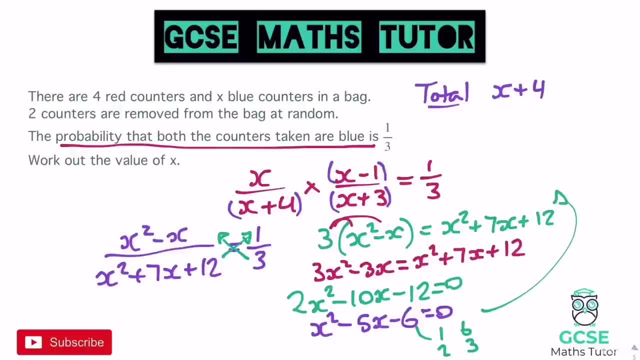 so this actually factorises. let's do it up here, open up our brackets and we want minus 5 in the middle, plus and negative 6 at the end. so the only option in there is going to be minus 6 and plus 1. that would allow us to get minus 5, so we'd have x minus 6 and x plus 1.. There we go, we've factorised. 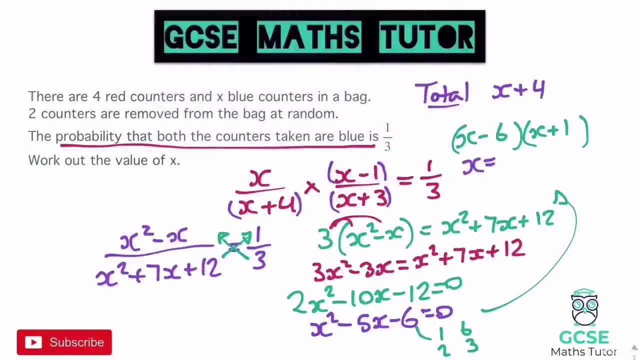 it. so we've got our two solutions there. so obviously you flip the sign, so x is 6 and for here x equals negative 1.. So what does this mean in terms of the question? Now, it said: work out the value of x. this is what we've been doing here: working out the value of x. 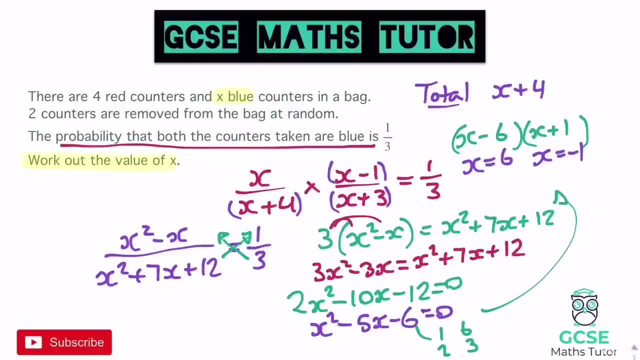 and x, there is the amount of blue counters. Now, there can't be minus 1 blue counters, can there? but there can be 6 blue counters, so it has to be the positive value there. x would have to equal 6 as our final answer, because we can't have minus 1 blue counters. so just something to be thinking. 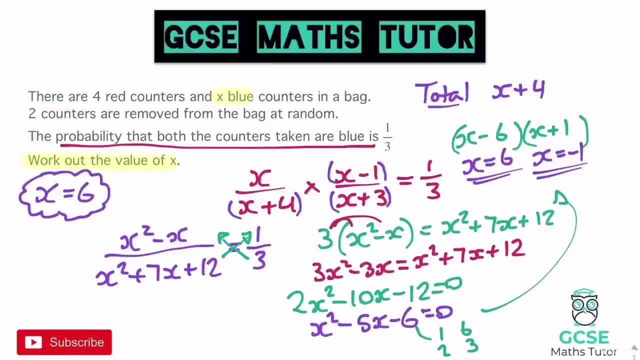 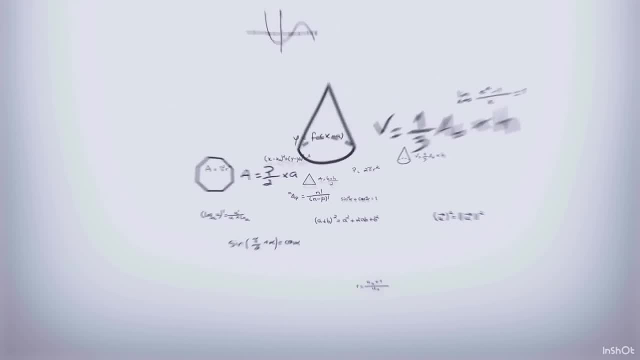 about there. Right, there we go, and that's the end of probability. Thanks for watching. 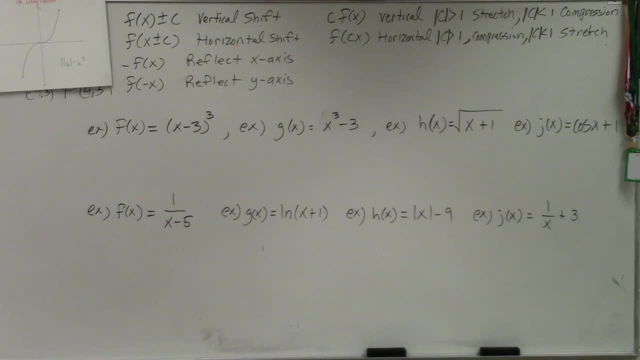 Understanding what we're doing. my recommendation to you is first identify the parent function, And the parent functions again are what's in your notes and what we have written up there on the board. I know this is kind of in the way a little bit.